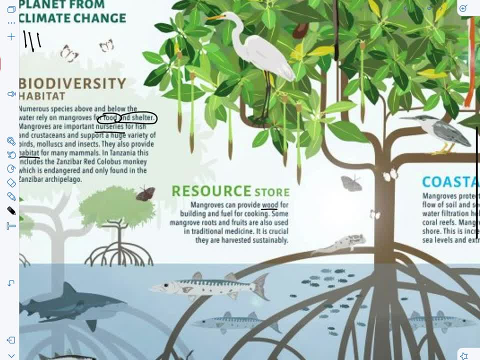 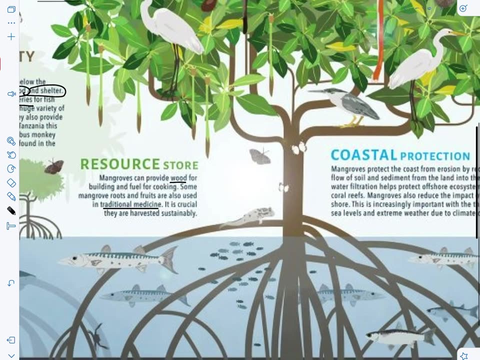 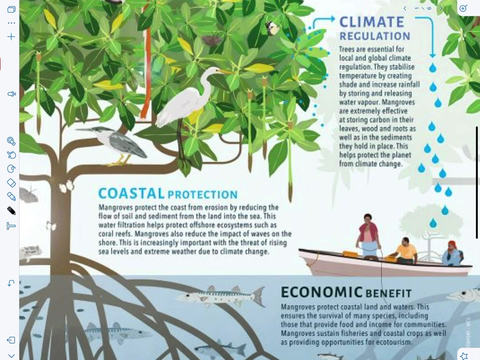 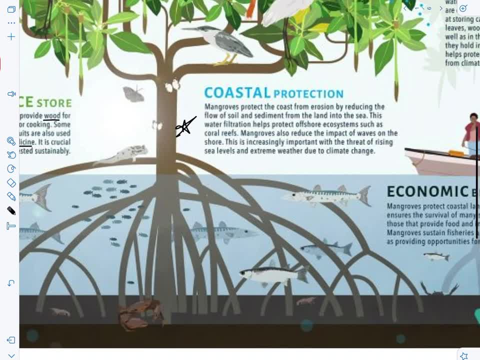 roots. here they're able to trap sediment by slowing down the water and then sediment will start to build up and it can actually build up the land, which is perfect for it because it needs soft sediment for its roots to grow into, so they protect the coast from erosion. 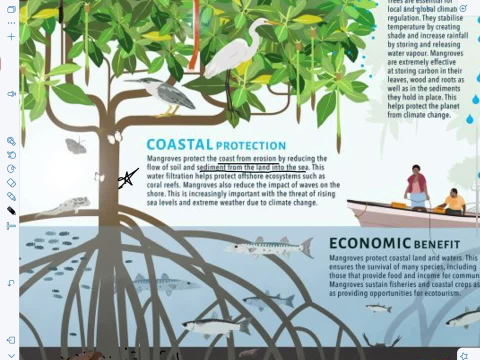 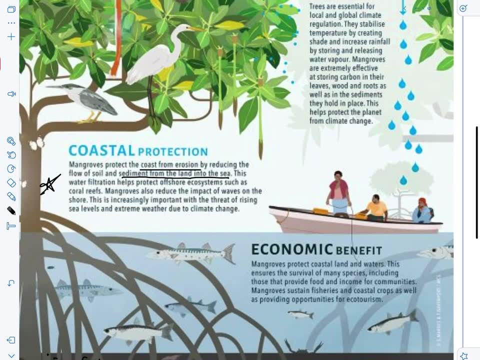 they reduce the sediment flow. um, they did it again. from land to the sea, so it's going to be a lot more abundant than they used to be. not great. they also can filter out water, because they'll filter out the did it again. mineral ions on cursors. y'all curses. 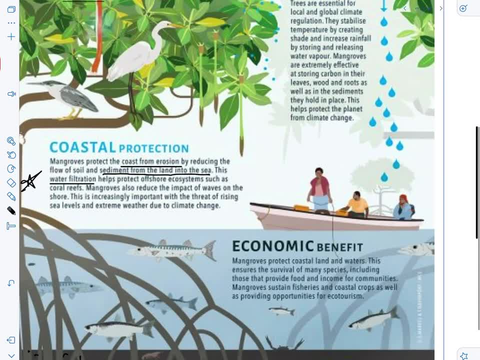 mineral ions and just excess nutrients, okay, and this will also again reduce the impact of waves that are on the shoreline. so it's gonna reduce the impact of waves that are on the shoreline, so it's gonna minimize coastal erosion and that is actually going to obviously be a really big plus for us. 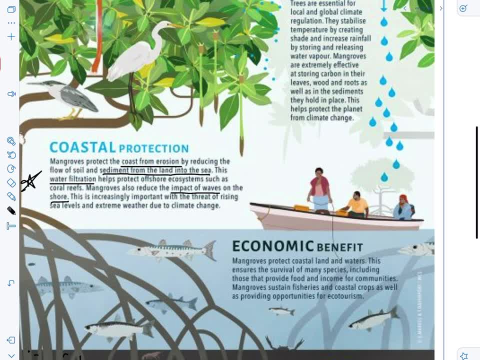 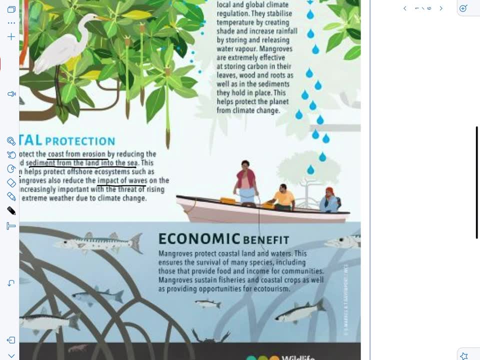 because it costs a lot of money when we have coastal erosion. what's not mentioned here? oh no, it is the climate one. there's economic benefits- economic benefits- and we're going to save money by not eroding our coast. we can also use the species that are there for food sources. 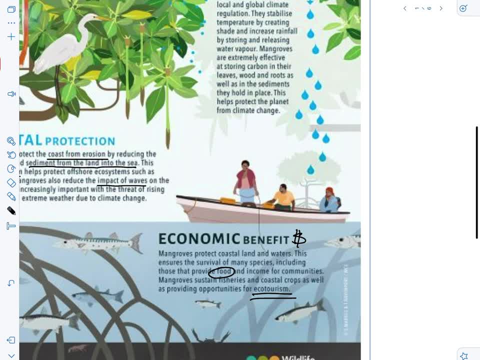 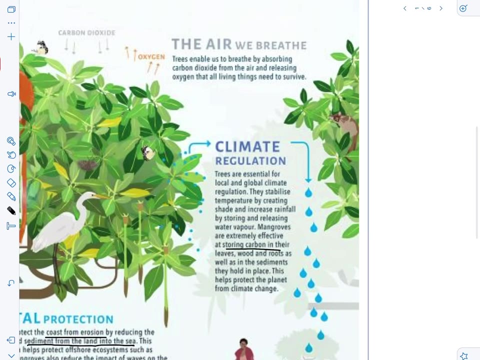 it provides ecotourism benefits. it's going to save us money through mitigating- helping to mitigate climate change, climate regulation. they absorb carbon dioxide from the atmosphere and they can store this carbon in their leaves and their wood, in their roots as well. the roots can store a lot. 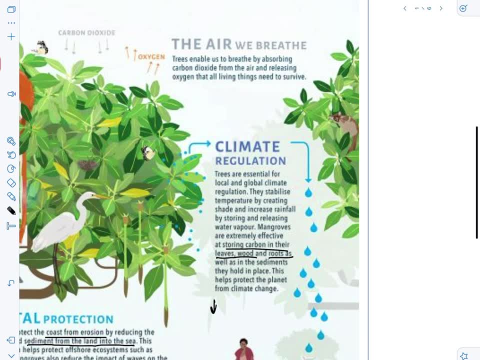 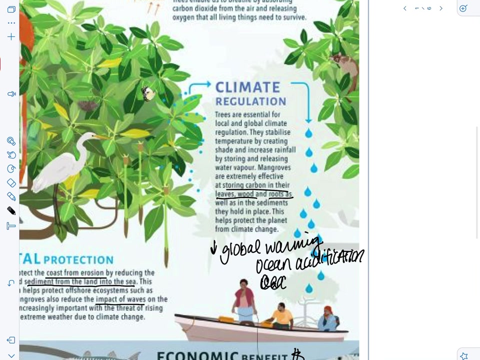 and so this will also help decrease global- just at the end- global warming and, of course, ocean acidification, which can cause erosion of organisms that have a calcium skeleton, a calcium exoskeleton. ocean acidification creates calcium, i was going to say calcium carbonate, no carbonic acid c-a-c-o-3. 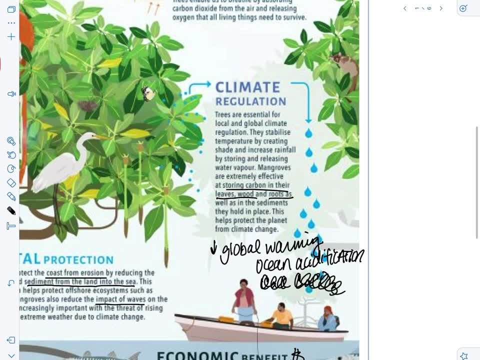 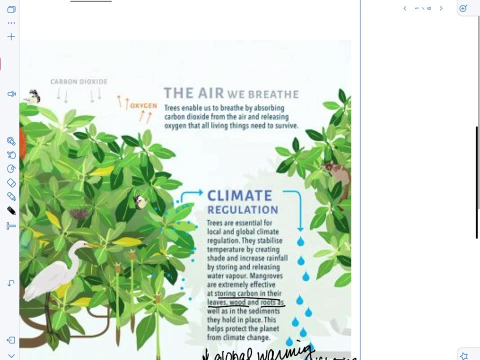 no, that's calcium carbonate, my bad h2o c-o-3. i knew that didn't sound right. okay, and then again, it provides. it does photosynthesis because it's a plant, so it's going to take out carbon dioxide from the atmosphere and synthesize. 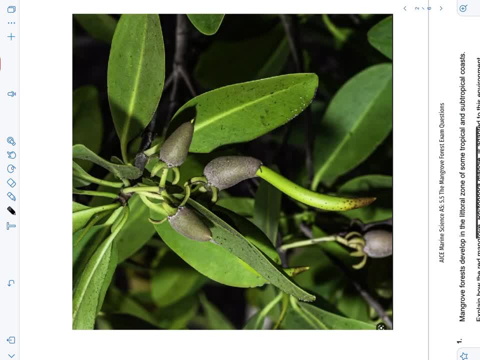 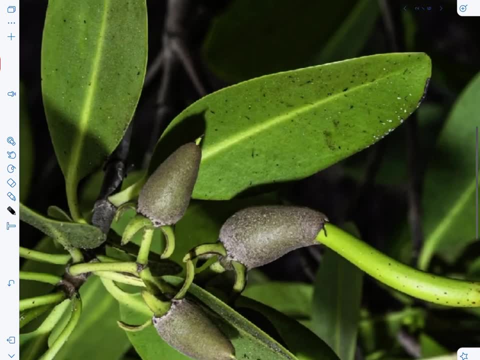 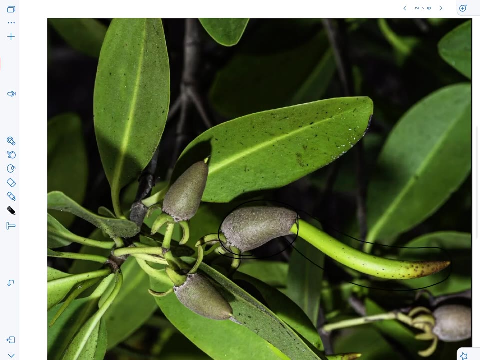 glucose and release oxygen, something that we're going to mention in the exam answer. that wasn't in the text, so it wasn't going to be in something of the note page that i made you is about their leaves. if we look at their leaves and you can see here this seedling. turning to the propagule, 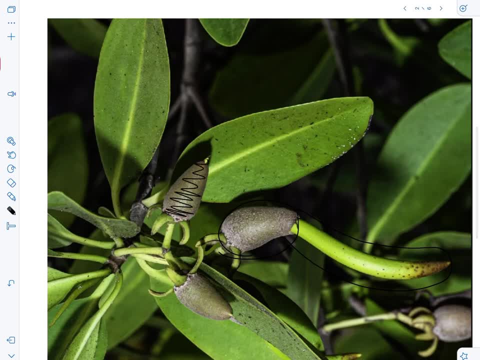 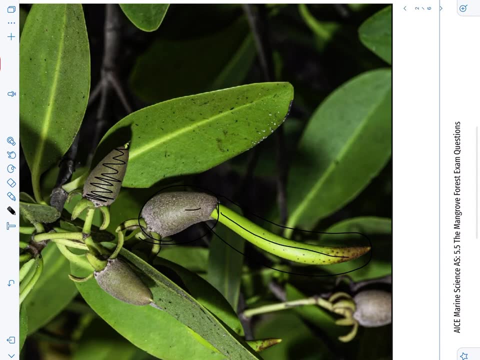 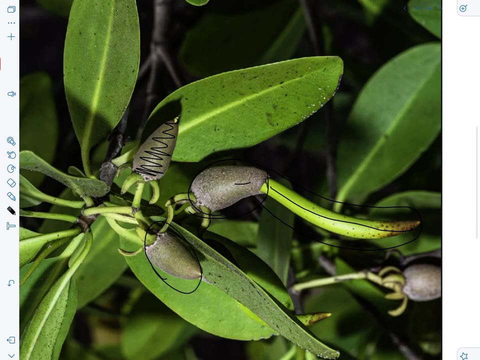 and these seedlings were a flower and it's a propagule, so it's literally growing from the seedling to the propagule off of the parent plant. it really couldn't survive if it dropped as a seed. it wouldn't be able to survive in the saline water, nor would it be able to be able to take root. just 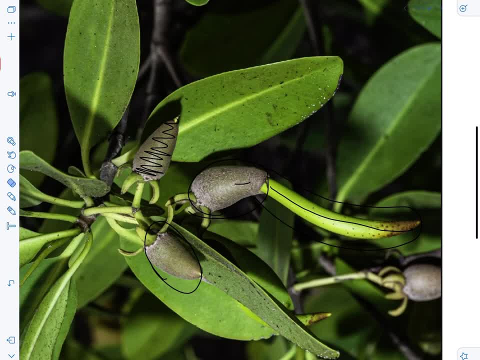 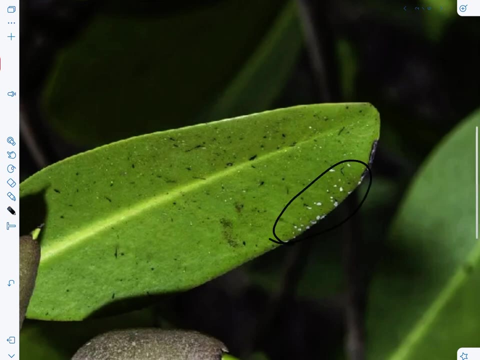 being the seeds, so the propagule is adapted for that. it will survive in the water as a normal seed help it float away from the parent plant. so it's not to compete with it, but something to notice. you have some salt excretion here and salt build up, and that's a good thing. that means it's not. 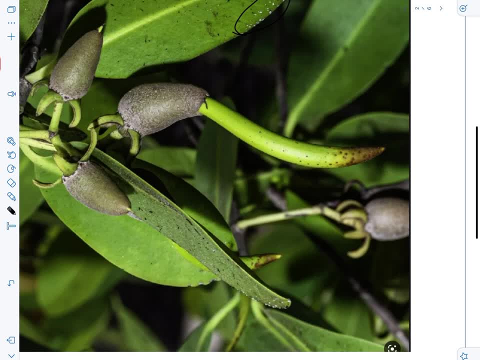 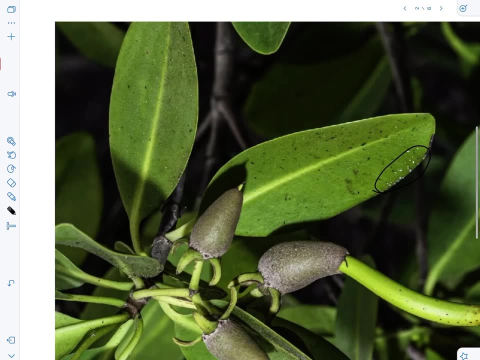 getting inside of the tissue itself, causing water loss through osmosis and you can see all the sediment that's on. there could have been windy, circumvent some wind erosion, but these leaves are, they're thick, they have a very waxy cuticle. cuticle is the outside covering of a leaf. um, they have a. there's some again. uh, like leather. 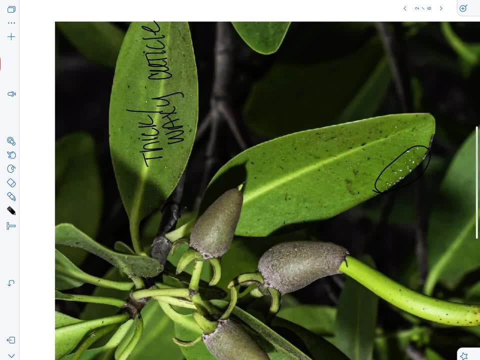 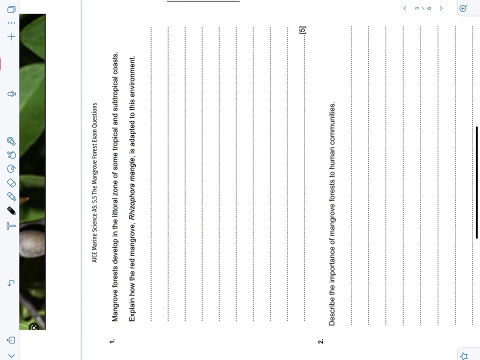 like structure, leather like structure, leather like texture. and so that is just going to aid the plant in not losing water. when it's in a salty environment, those leaves are very tough, okay. so this first question: mangrove forest developed in the littoral zone, the vital zone? is also called the intertidal zone, so you're gonna have salty water, but it's estuarine, i'm gonna spell it right. means you have fresh water input from a river in salt water, from the ocean of some tropical and sub-tropical coast. remember they grow between 25 north to 25 south. they grow best 25 degrees. 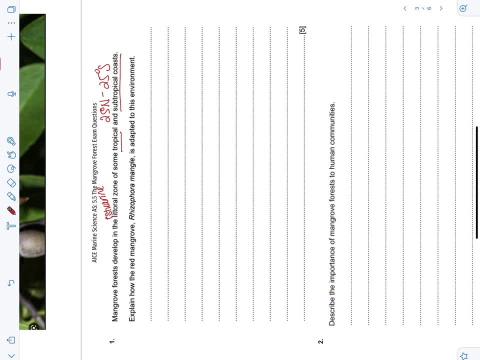 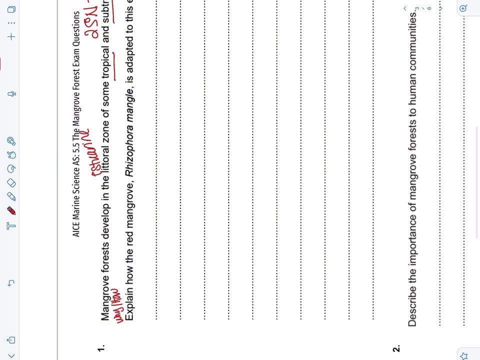 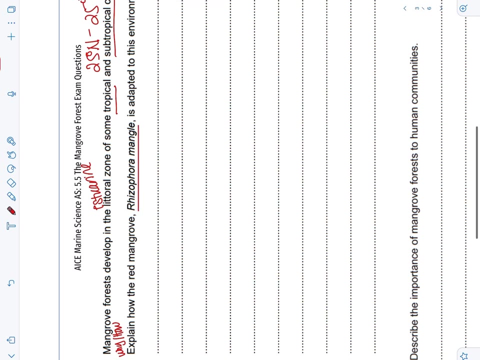 north, 25 degrees south. they grow best, grow best there, so you need warm temperature year round. explain which is why and how the red mangrove rhizophora mangle- notice it's in italics this is its scientific name or its species name, genus, and then species is adapted to this environment. so we need to talk about. 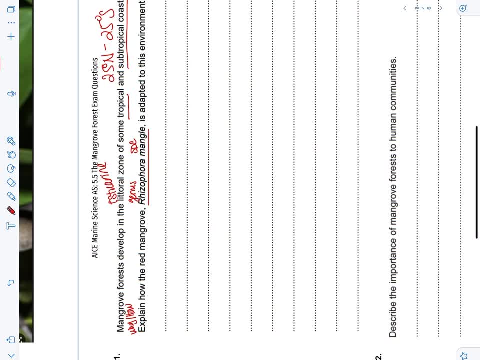 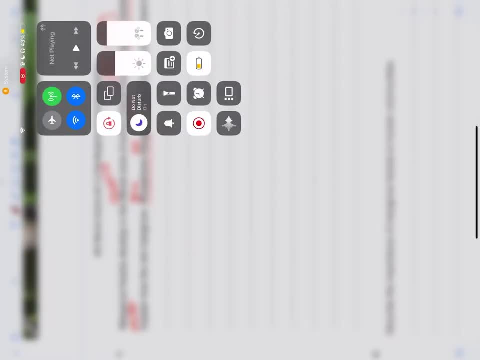 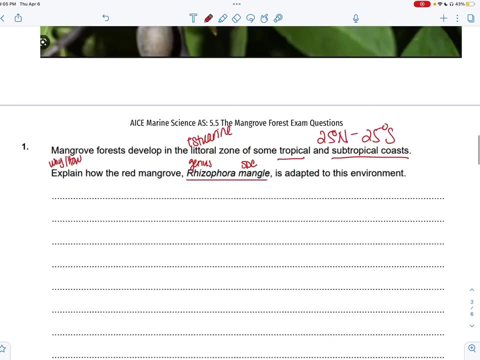 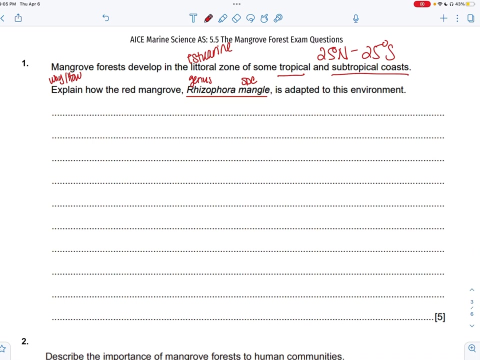 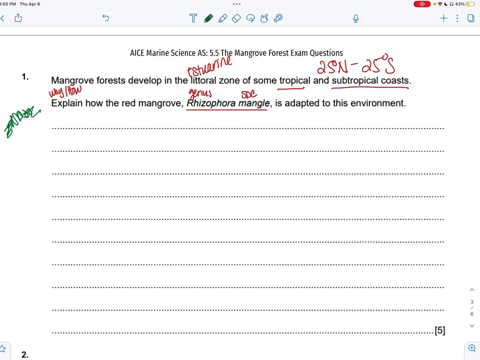 the adaptations of it, living in the littoral zone or the intertidal zone, in tropical and subtropical areas. i just might prefer this better. okay, all right, so if we want to think about just top down with the plant, okay, so we have the leaves. this is just gonna be a fabulous sketch. I'll 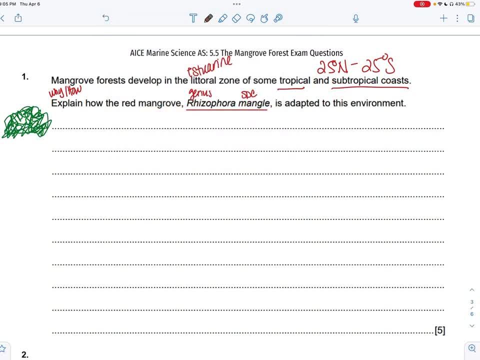 have to talk about that. and then it's fabulous roots, the prop roots and what else they have on them. are there, sweet little babes, the little propagules? and something else we can mention are the lenticels that are on the top of the roots, and again they close the. 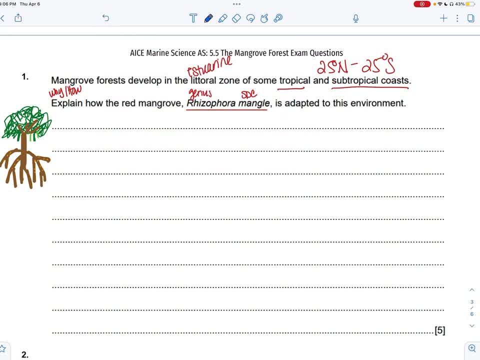 leaves sounds so fun. we have another giant thing that we see is more beautiful when they grow up up, whenever they get inundated with water from storm surge or really high spring tides- your high tides, okay- and so a lot of it stays submerged, but there are some that are on the top of the water. 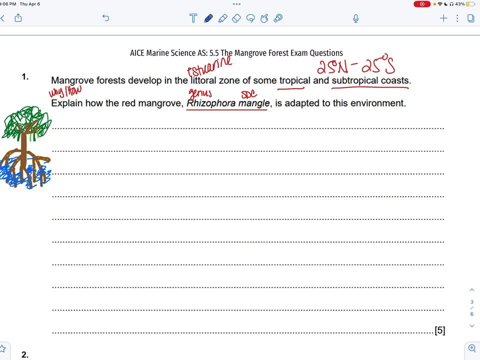 that stick out and we've all seen that because we live by them and that's just going to aid them in absorbing oxygen from the atmosphere. so we'll want to think about this top down so we can get to writing about it, okay, um, starting at the top, then we can talk about their leaves, and this is something that 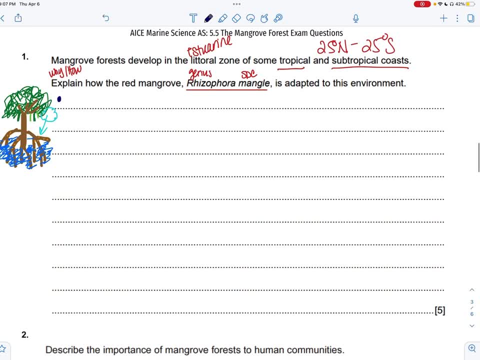 though it's expected to be answered on the exam question, i can tell you it is not put in the syllabus, nor was it put in the textbook. so another emphasis on going through exam answers is really important. so they have tough, thick- it's referred to as leathery leaves and we're looking for the explain command words so that. 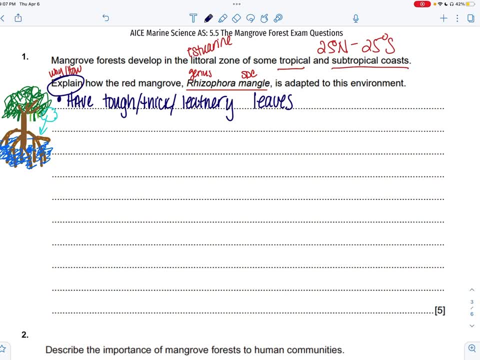 really is just a statement. we need to explain it. this will be to reduce evaporation. just see, explain moving down their their roots. they have prop roots and we got to consider what their substrate is like. they're not an iraqi substrate. sometimes they're in a muddy area, where they're in an area with really fine sediments, which is easily 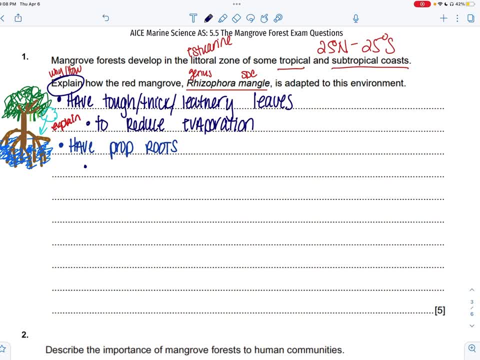 erodible and if it was just one, like one wooden structure holding up the tree, and then you had a lot of erosion, a lot of water erosion that's gonna. that could definitely cause it to erode away and get dislodged from the sediment. but this plant has multiple anchors, so even if one 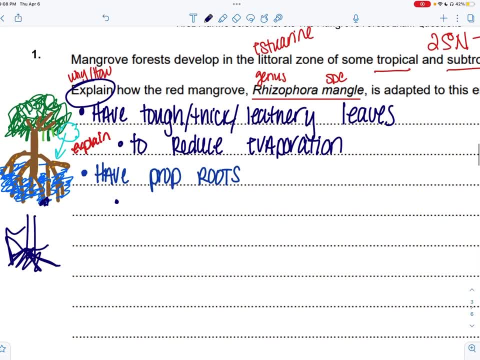 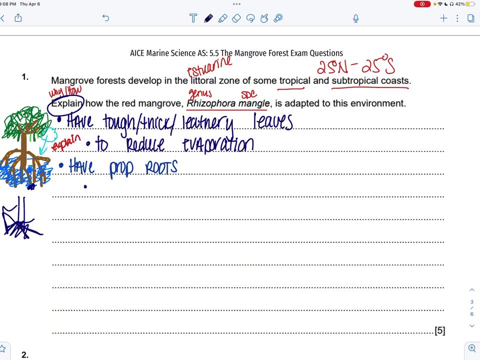 kind of loses the sediment around it. it's it's not going to be a detriment to the plant and so this is the okay statement: prop roots and then explain: to provide stability or Anchorage for unstable substrates. something else we referred to as an unstable substrate was: 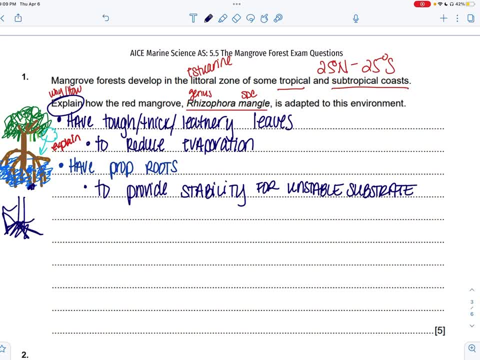 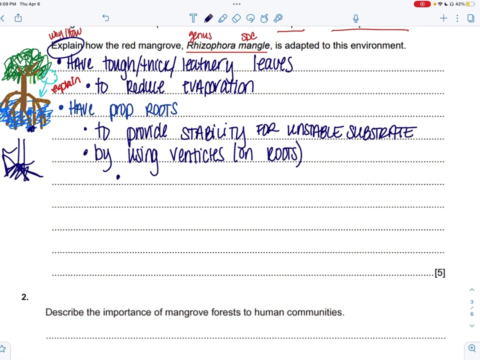 the sandy shore, but we're not doing the roots yet. there's also more adaptations there by using the venticles on the roots. again, these are on the outside of it that are above the water line. oxygen from the atmosphere- it's absorbed, okay, and then why does that have to happen? like, what's the adaptation for that? 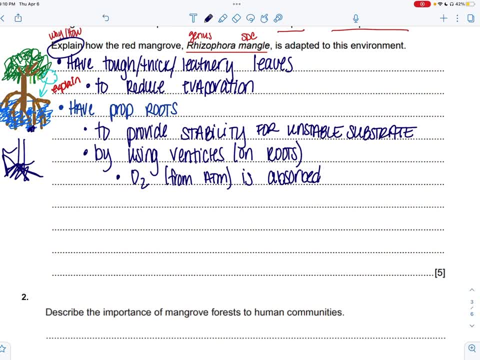 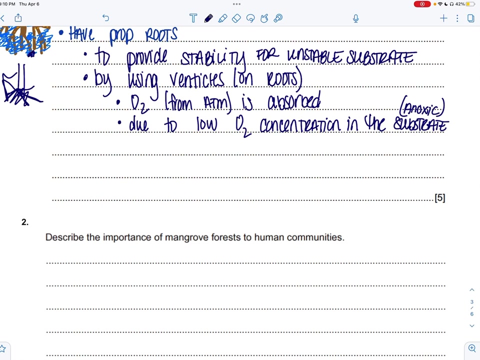 if they're absorbing it from the atmosphere, that means that there must not be some in the habitat. the roots are actually in. this is due to low oxygen concentration in the substrate, or you can refer to this as the anoxic substrate. oxic refers to the amount of oxygen and meaning something negative or not. so anoxic, not oxygen. 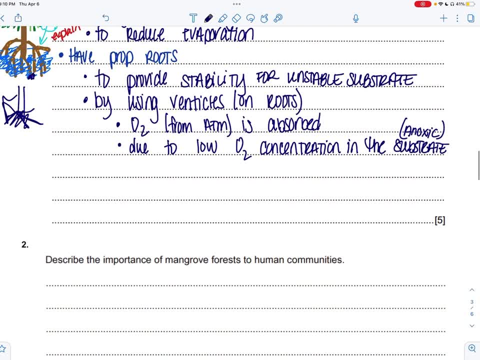 almost through. we're not done with the roots yet. but the roots have salt exclusion. I think the video. I said salt seclusion. they seclude themselves from the salt. they exclude the salt. roots can exclude salt. why is this important? from the sorry high salinity content. 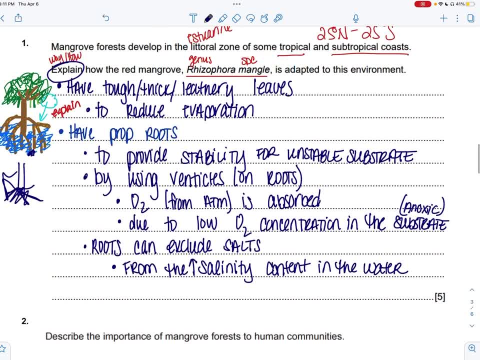 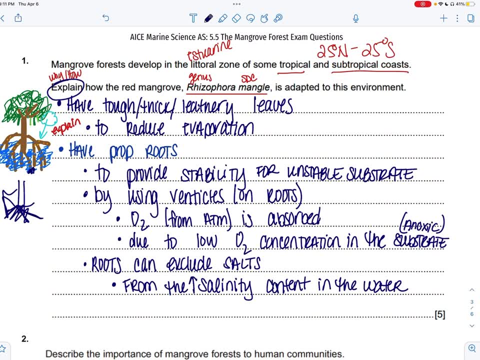 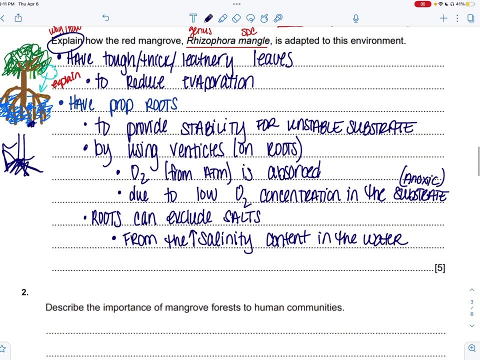 in the water? if anyone's looking for this question, it is from the specimen paper one specimen paper, one for the 2022 syllabus. if they're not in my class, almost done- and then if they're adapted, that environment it's not just that plant, it's going to be that plant. 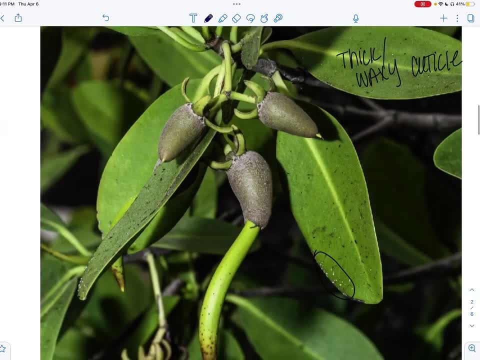 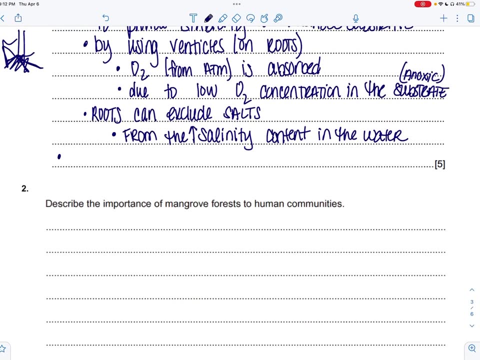 and its future plants. so we need to talk about the sweet little little offsprings, little propagules, all right, mangroves, um, perform, i don't think perform- and i just said them again, i'm so sorry- i think perform is like the good word for it. mangroves have maybe viva, which means life. 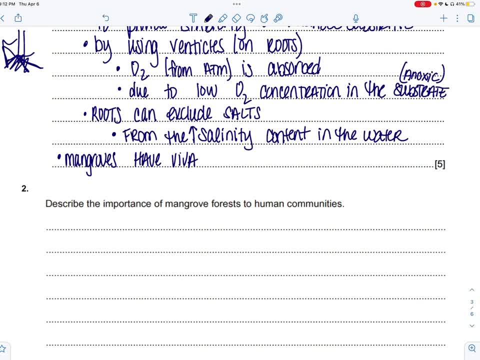 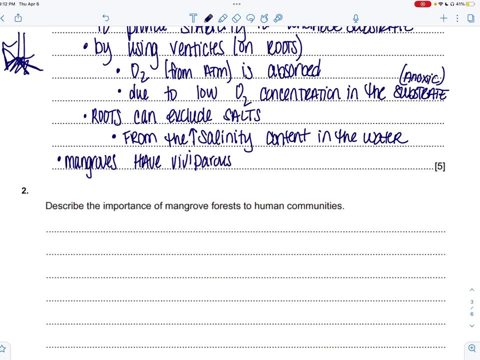 by this or risk. sorry, not viva vb. that sounds better if you put methods at the end in parentheses. it's not exactly part of the exam answer, but mentioning that they have viviparous reproduction methods or they do viviparous reproduction um, which essentially is inside, i'm saying that that these propagules, many plants will. 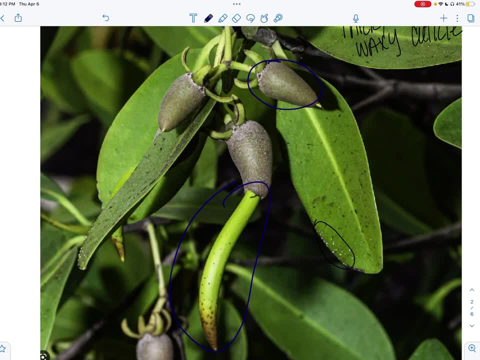 drop their seeds. sometimes they'll drop it in the form of a fruit and then the seeds are on the inside, so animals will eat it- walk away from the parent plant, excrete it somewhere else, and now that seed is going to be growing further away from the parent plant. but if they just drop, 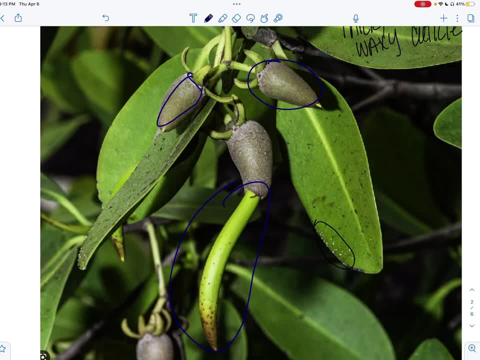 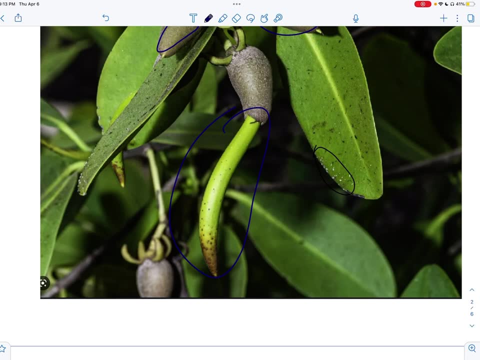 these seeds. like i said, these seeds wouldn't survive in the salt water, so they spend some time getting nourishment, getting nutrients, getting fresh water that's been filtered through the parent plant. again, that's something that mangroves can do. they can filter through the water they can. 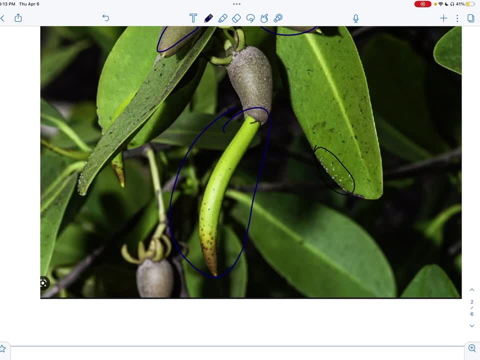 filter out the excess sediments and and salt from the water. so this propagule right here is able to gain the nutrients that it would typically get on its own if it was in like a freshwater setting or a terrestrial setting, land setting. but because it's in a salt environment, it 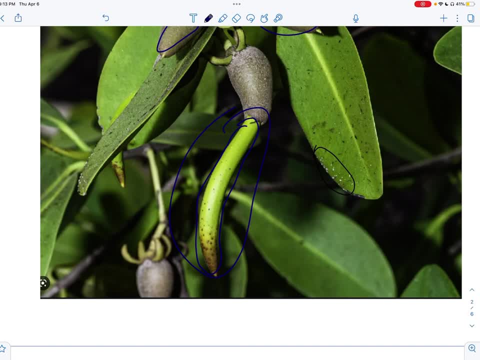 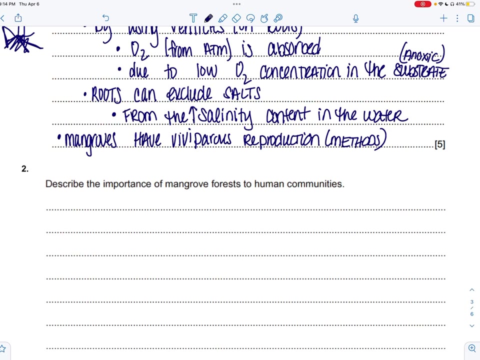 has to spend a lot of time developing itself to be able to be freed away whenever it's a little bit bigger and it can float through the ocean and not die due to water loss. so viviparous reproduction methods by using propagules. another mark with that: viviparous reproduction. 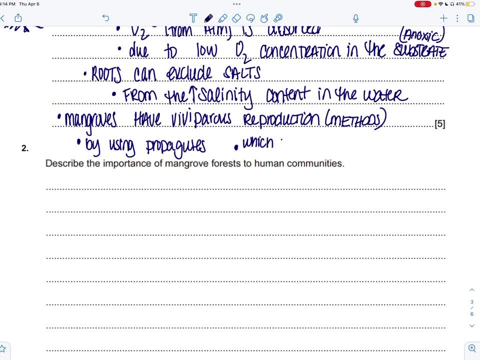 regarding the propagules which float upright growth starts and they can float for up to a year on average about 40 days. they'll float in the ocean. they'll float away on the surface currents away from the parent plant. growth starts when propagule settles in a 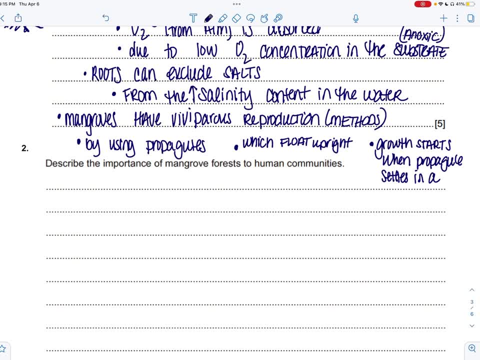 um sediment-rich substrate or a suitable substrate. i just don't love the use of suitable, because then you're not really describing what's suitable. i'm trying the word a substrate with fine sediments, because it can't be a rocky substrate, okay, and i'm actually gonna crop this answer and move it so it's not in the way. 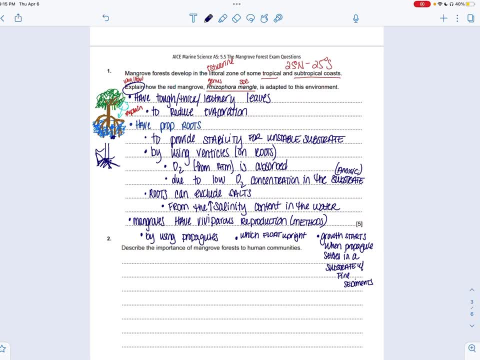 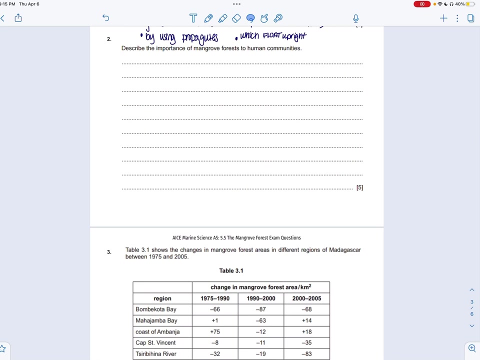 okay, so that one top to bottom is all the answers. She's just five marks. Move this out of the way. Okay, now discuss the importance of mangrove forests to human communities So you can reference what you have on your note page. I think the only thing. 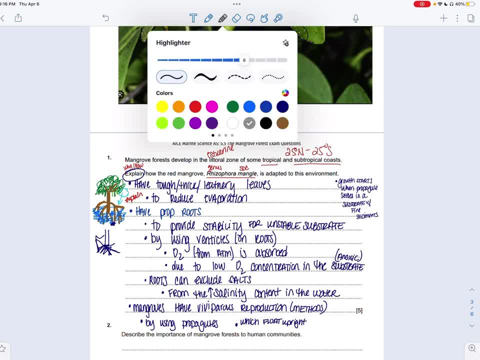 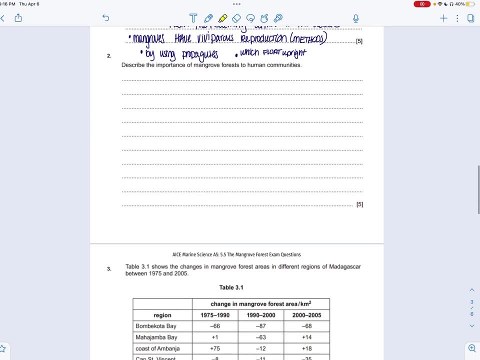 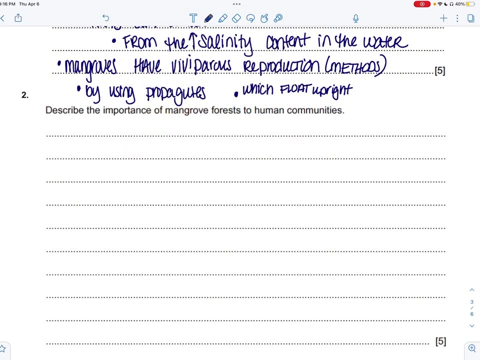 that was not on your note page from this question was this first one, about their leaves, But now you have it. Discuss the importance of mangrove forests to human communities. It's how they support humans. This would be a lot of that economic benefit that we 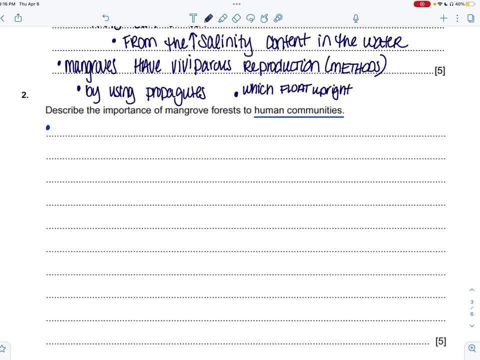 mentioned and what I just mentioned, the beginning of this. Okay, we can first talk about that. we get food sources from there. The food sources are going to be fish, shellfish and shellfish species. So what do the mangrove forests do that is going to aid our food sources. It's going to help us. 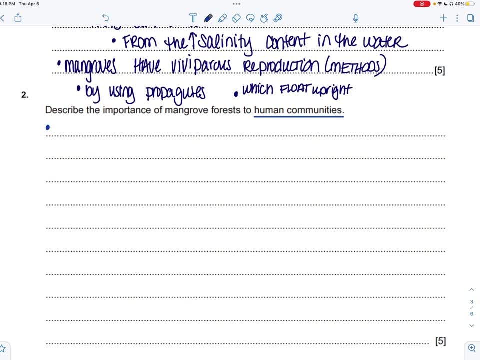 be able to get those food sources. So we could start with that one. Mangroves are a habitat for human and this is also in parentheses in the mark scheme, Just so you have the more specifics Food sources or food species They are. 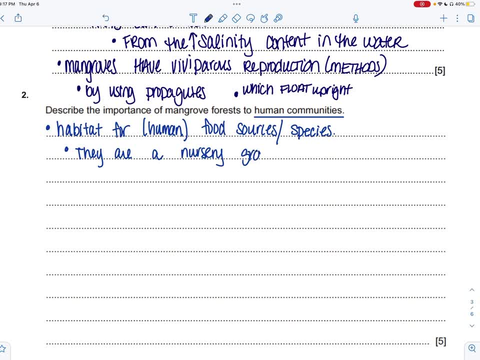 a nursery ground, And that's for the juvenile species. mangroves are also a breeding ground for our food species. within the statement of it being a nursery ground, it's a nursery. it's gonna be for a younger species, so we refer to them as juveniles. juvenile species use proper roots of the 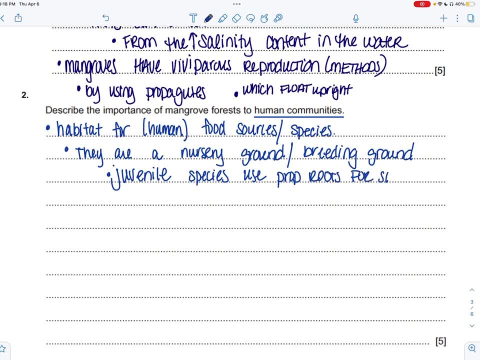 mangrove for shelter, and so with that, as a juvenile species, they're going to be able to survive because they are sheltered within the proper roots properties will also give them oxygen for respiration. they are also gonna be able to supply, just being by the plant in general, organic material as it's a. 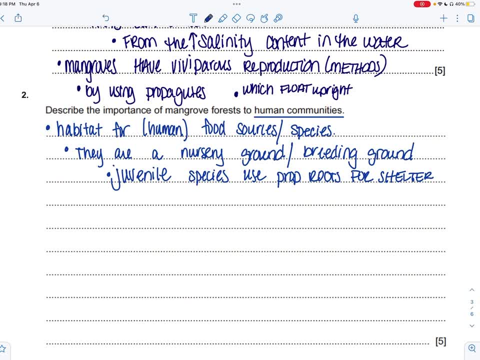 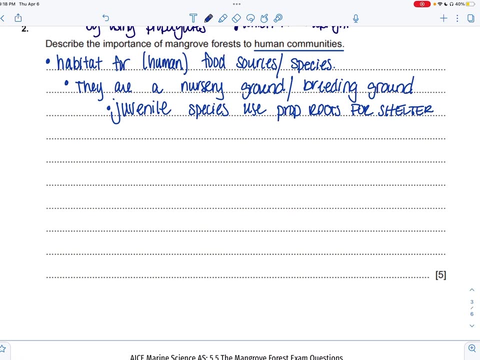 producer, so it's a really great trophic level one organism anyway, and that is going to aid in our food species, our future food source, growing and just thriving. okay. another one: mangroves provide or allow for ecotourism or even just tourism industry anytime anybody's you know coming to Florida or in our area and they 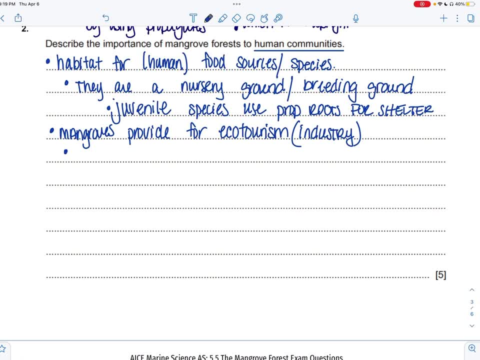 go in a dolphin tour or they go into kayaking or stand-up paddleboard- things like that- within the river. that is supporting ecotourism, because they are inadvertently also learning about the ecosystem, gaining a deeper appreciation for it. it's hiring local community members to make sure that they're getting. 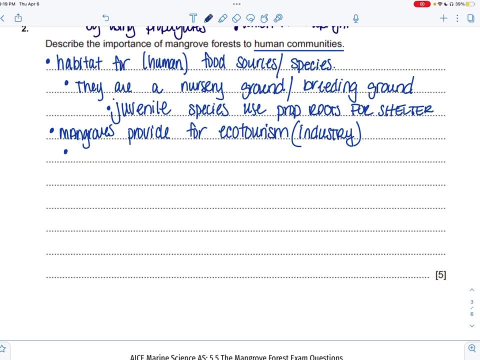 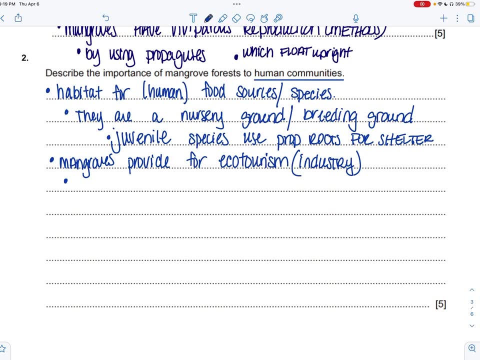 members and then adding money back into our community. all right, don't need this another, really big one. for us, it offers coastal protection from waves and storms. you're mentioning that. they help reduce erosion, their timber or lumber sources, they are fuel sources and, again, in a reference to the biodiversity that you guys went through last week, 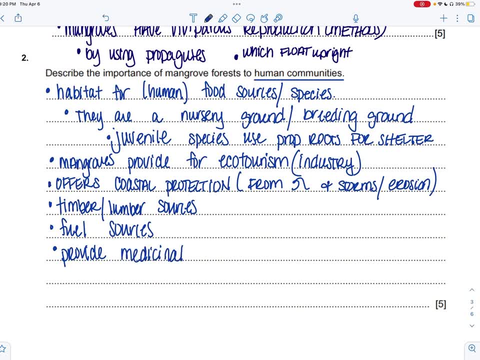 they provide medicinal products or provisions, and one that is detrimental globally, that they help human communities with mangroves. mangroves- mangroves- decrease co2 through photosynthesis and, within that same climate change or mentioning of carbon dioxide, they're going to decrease global warming. 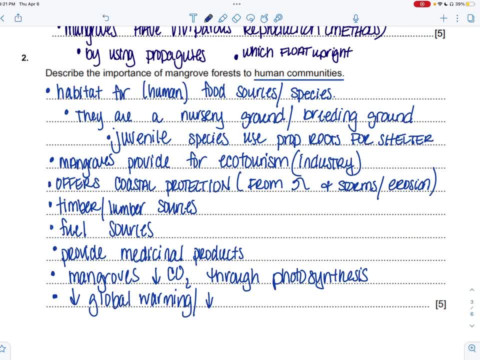 or you could say decreasing, not going down, or. or you could say decreasing, not going down, or. or you could say decreasing, not going down, or lowering but decreasing would be a better lowering, but decreasing would be a better lowering, but decreasing would be a better one. if you're talking about a rate, 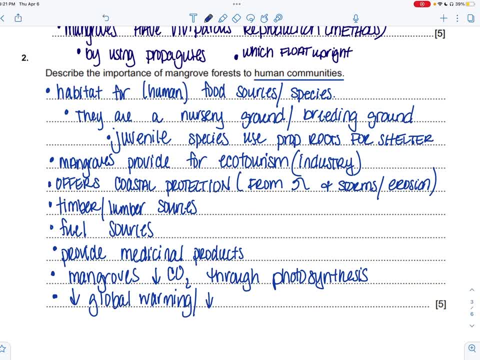 one if you're talking about a rate one, if you're talking about a rate decreasing um ocean acidification, decreasing um ocean acidification. decreasing um ocean acidification because if they're taking in the co2, because if they're taking in the co2, because if they're taking in the co2, then it's not getting dissolved in the. 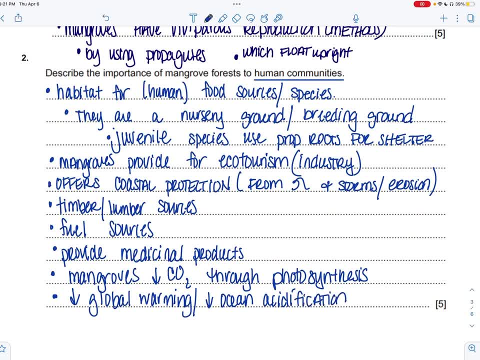 then it's not getting dissolved in the, then it's not getting dissolved in the ocean- ocean- ocean. that also will affect our food sources. if that also will affect our food sources, if that also will affect our food sources if shellfish are one of them. shellfish are one of them. 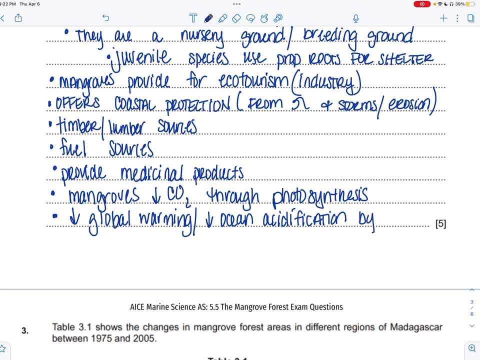 shellfish are one of them. ocean acidification, ocean acidification. ocean acidification by, by, by acting as a carbon sink or carbon storage. there's the difference between a carbon. there's the difference between a carbon. there's the difference between a carbon sink and a carbon source. 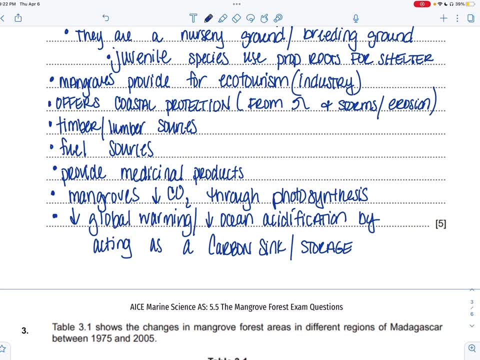 sink and a carbon source. sink and a carbon source: um a source is going to be where um a source is going to be, where um a source is going to be, where something is coming from like its source. something is coming from like its source, something is coming from like its source. so, 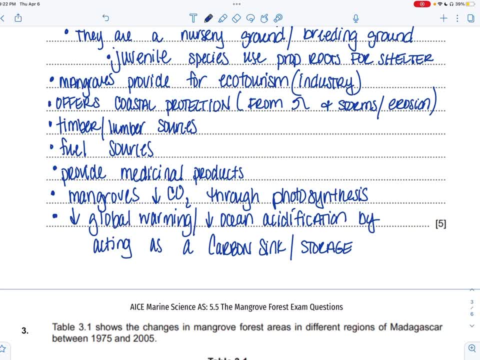 so. so the sink is going to be if you turn on. the sink is going to be if you turn on, the sink is going to be if you turn on the sink, the sink, the sink. water goes down into the sink, a sink. water goes down into the sink, a sink. 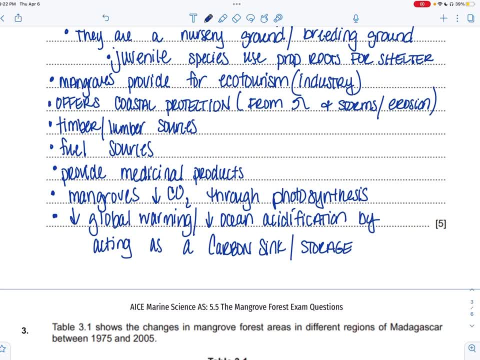 water goes down into the sink- a sink. the sink is where something is going to get stored, is where something is going to get stored, is where something is going to get stored and it gets like sunk into. okay, so that one's just about humans. okay, so that one's just about humans. 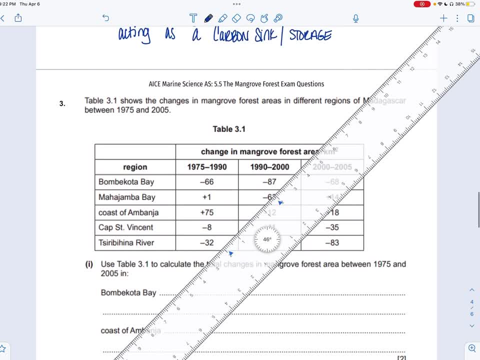 okay, so that one's just about humans. some math? oh hello ruler. how do i get some math? oh hello ruler. how do i get some math? oh hello ruler. how do i get rid of the ruler? rid of the ruler. rid of the ruler. just move it out of the way. 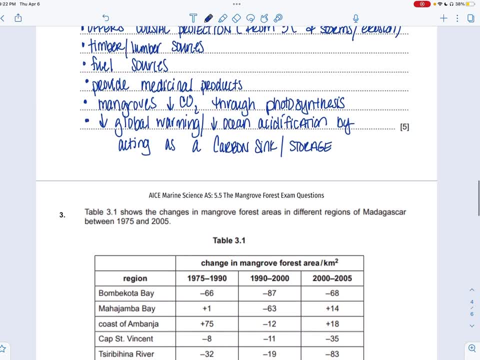 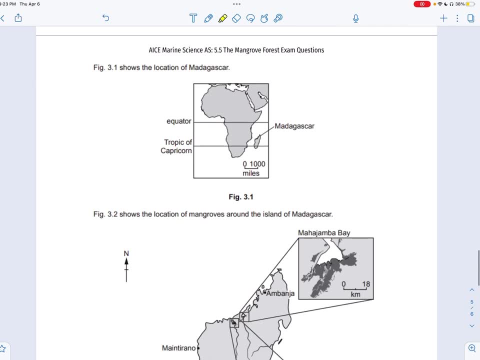 get out of here. okay, all right, table 3.1 and this question. all right, table 3.1 and this question. all right, table 3.1 and this question actually goes, actually goes, actually goes with this one, but the way that it was with this one, but the way that it was. 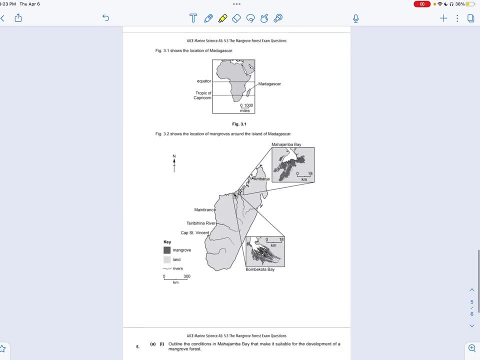 with this one, but the way that it was printed i wanted you to see printed. i wanted you to see printed. i wanted you to see the figure that they gave you and then the figure that they gave you, and then the figure that they gave you and then the questions that associated with it. i the questions that associated with it. i the questions that associated with it. i want you to see it together. so i did want you to see it together. so i did want you to see it together, so i did switch up the numbers a bit. switch up the numbers a bit. 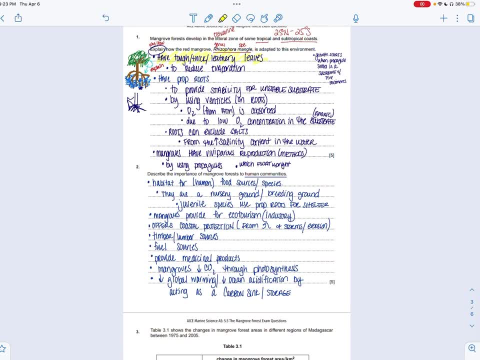 switch up the numbers a bit. um sorry, i didn't mention for people who: um sorry, i didn't mention for people who- um sorry, i didn't mention for people who are not, are not, are not my student right now, but maybe you're my student right now, but maybe you're. 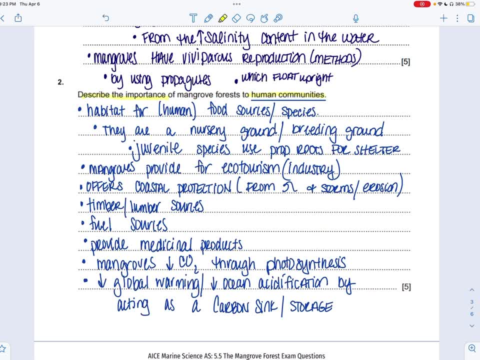 my student right now, but maybe you're not. i believe it's paper one and it's not. i believe it's paper one and it's not. i believe it's paper one and it's the very last question, the very last question, the very last question with paper 11 rather, and actually paper. 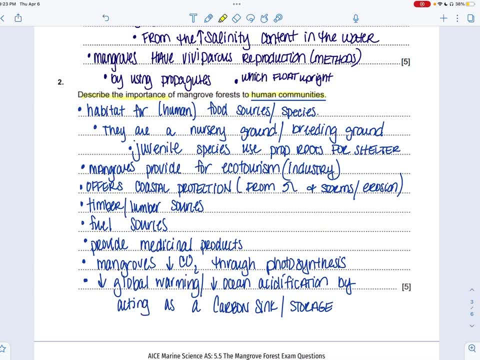 with paper 11 rather and actually paper. with paper 11 rather and actually paper. 11, 12 and 13 were all identical. 11, 12 and 13 were all identical. 11, 12 and 13 were all identical. um, it's the very last page. 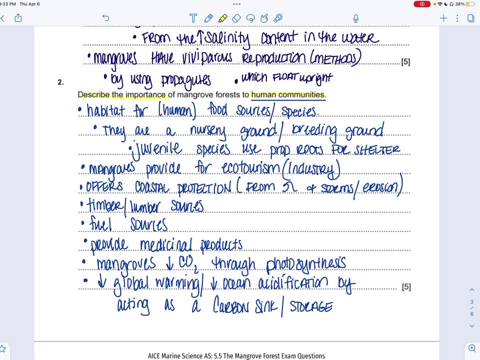 question 6b. now, the remaining of these are going to now. the remaining of these are going to now. the remaining of these are going to be from, be from, be from what my students took last year, the what my students took last year, the what my students took last year. the paper 11. 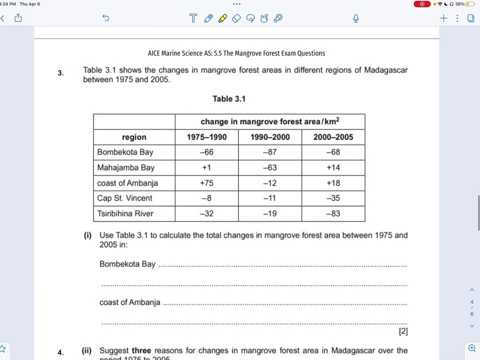 paper: 11 paper. 11 may june 2022. may june 2022. may june 2022 again. the other one was that number two again. the other one was that number two again. the other one was that number two on here was from: 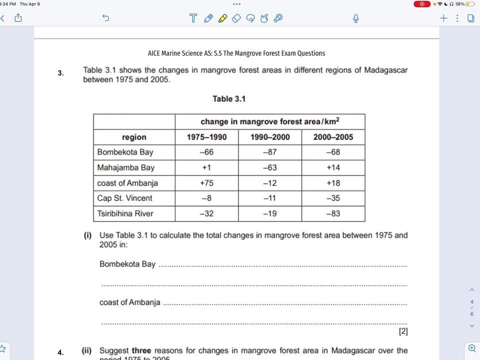 on. here was from on. here was from october november 2022. um all the papers, october, november 2022, um all the papers. october, november 2022. um. all the papers were the same, were the same, were the same. that was the paper ones, the first. 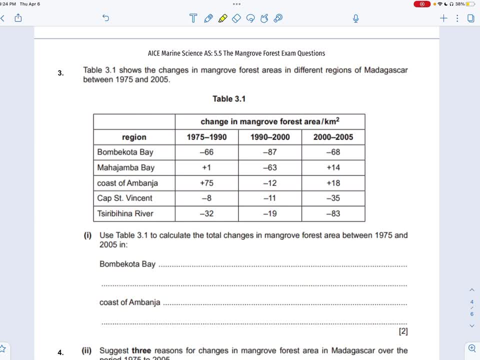 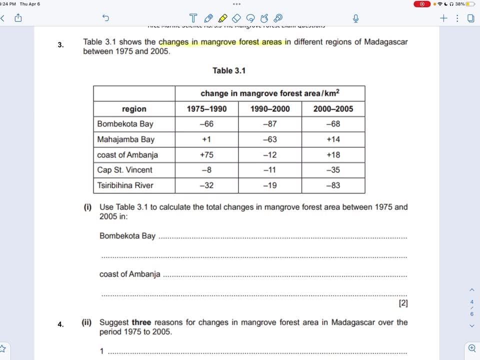 that was the paper ones. the first, that was the paper ones. the first question is from. question is from question is from the specimen paper one. okay, so we're looking at changes in the. okay, so we're looking at changes in the. okay, so we're looking at changes in the mangrove forest areas. 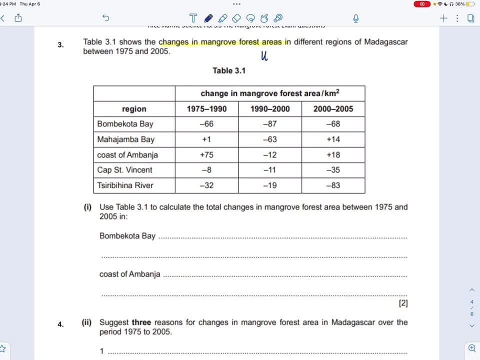 mangrove forest areas. mangrove forest areas. so we're probably going to be needing to. so we're probably going to be needing to. so we're probably going to be needing to. look at an area unit. consider units for. look at an area unit. consider units for. 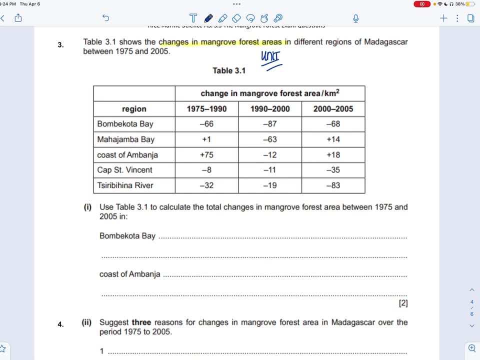 look at an area unit, consider units for this, this, this in different regions of madagascar, in different regions of madagascar, in different regions of madagascar between 1975 and 2005.. between 1975 and 2005.. between 1975 and 2005.. so here are your regions. 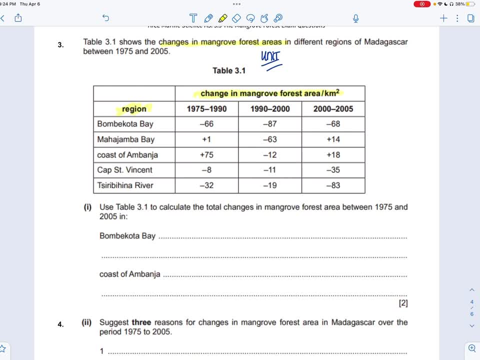 and then the changes in the forest area, and then the changes in the forest area, and then the changes in the forest area. there's your unit measured in kilometer. there's your unit measured in kilometer. there's your unit measured in kilometer squared square kilometers. 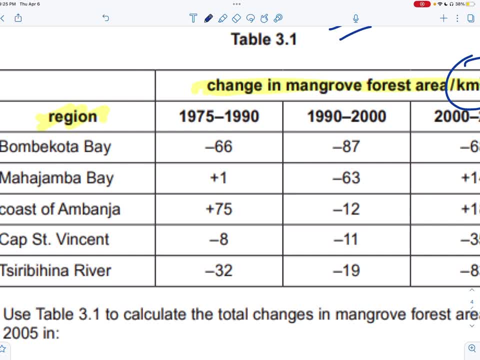 okay. so the way we can read this is okay, so the way we can read this is okay. so the way we can read this is like, like, like from 1975 to 1990, from 1975 to 1990, from 1975 to 1990, except 15 year period. 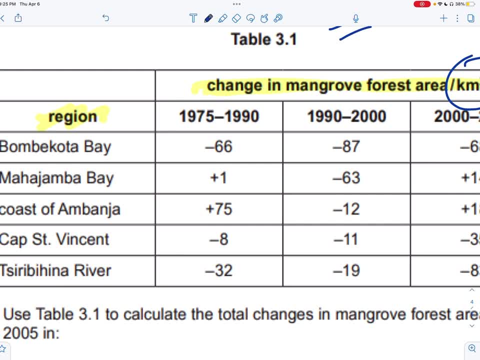 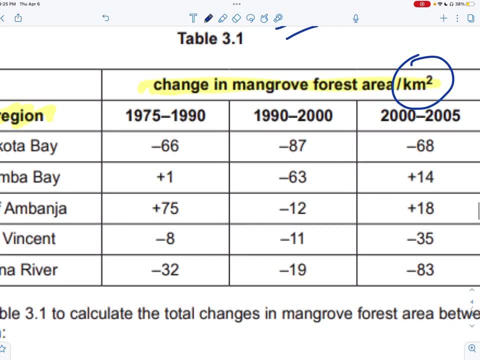 bomba kota, bomba kota, bombacota bay, bombacota bay. bombacota bay lost 66 kilometers square kilometers. lost 66 kilometers square kilometers. lost 66 kilometers square kilometers. and then, in 1990 to 2000, just in that. 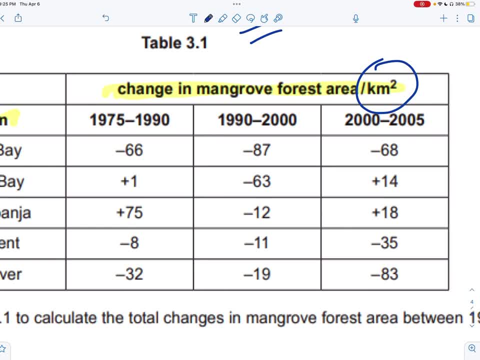 and then in 1990 to 2000. just in that, and then in 1990 to 2000. just in that 10-year period, they lost 87 square 10-year period. they lost 87 square 10-year period. they lost 87 square kilometers. and 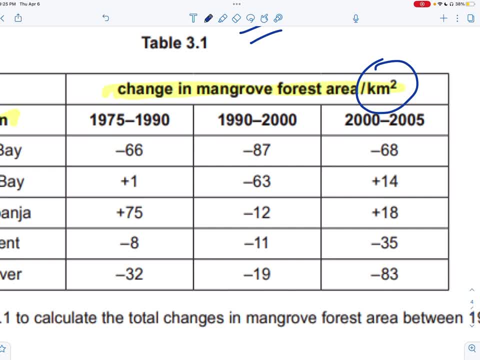 kilometers and kilometers, and then in a five-year period, they lost. then in a five-year period, they lost. then in a five-year period, they lost a 68 square kilometers. so the rate of a 68 square kilometers, so the rate of a 68 square kilometers. so the rate of loss. 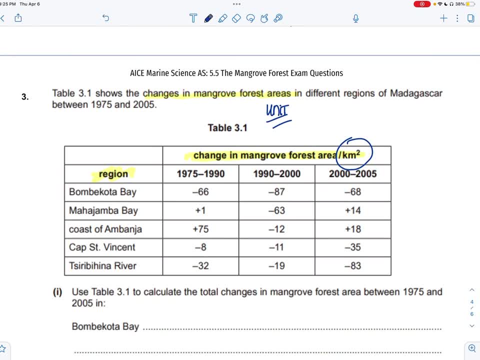 loss. loss- it's definitely increasing for sure. it's definitely increasing for sure. it's definitely increasing for sure. so that's how we, that's how we read it. so that's how we. that's how we read it. so that's how we. that's how we read it. use the table calculate. 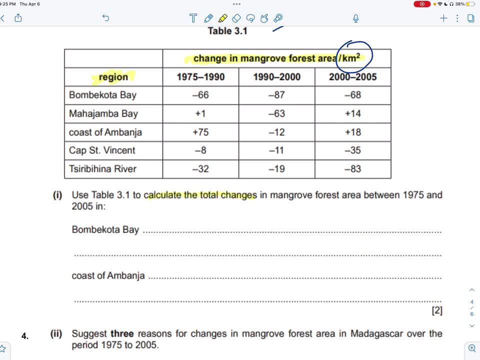 use the table calculate. use the table calculate the total changes, so gain or loss. the total changes, so gain or loss. the total changes, so gain or loss in mangrove forest area between 1975. in mangrove forest area between 1975. in mangrove forest area between 1975 and 2005.. 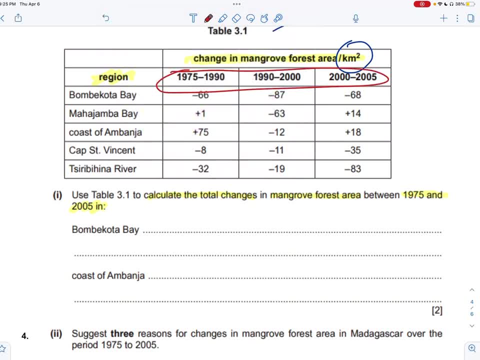 and 2005.. and 2005.. so we need to take, we need to take in, so we need to take, we need to take in, so we need to take, we need to take in account, account, account, um, all of these values. so, starting at, 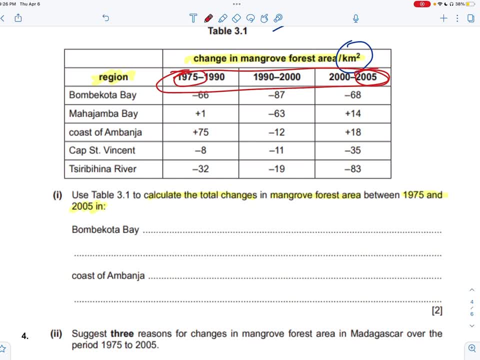 um all of these values, so starting at um, all of these values, so starting at 1975, ending at 2005.. 1975 ending at 2005.. 1975 ending at 2005.. the first one is bombacota. i'm. 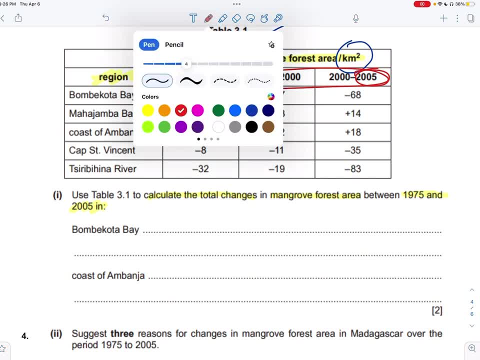 the first one is bombacota. i'm the first one is bombacota, i'm sure, i'm saying it, sure, i'm saying it, sure, i'm saying it, not correct. total changes, so it's a number. so total changes, so it's a number, so. 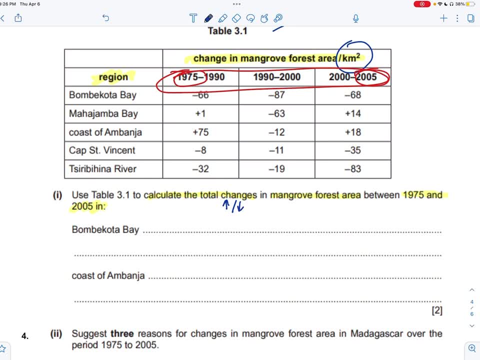 total changes. so it's a number. so remember it can increase, or it could remember it can increase, or it could remember it can increase or it could decrease, or i guess it could stay the decrease, or i guess it could stay the decrease, or i guess it could stay the same. 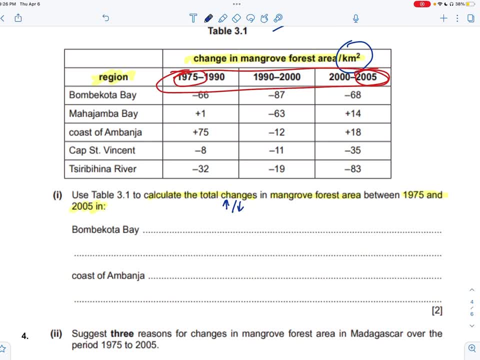 same same. mama kota bay, so between 75 and 90. mama kota bay, so between 75 and 90. mama kota bay, so between 75 and 90. it lost 66, it lost 66. it lost 66 square kilometers. this is not the answer. 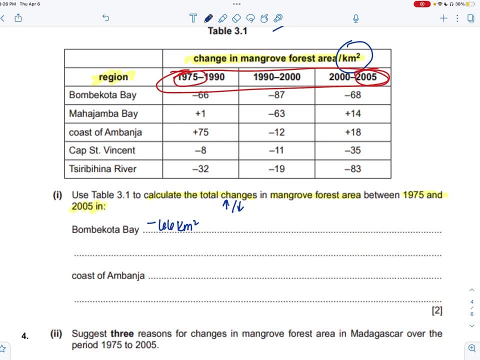 square kilometers? this is not the answer. square kilometers? this is not the answer. i'm just showing you that, the word for, i'm just showing you that, the word for, i'm just showing you that, the word for it, it, it, and then 1992 000 it. 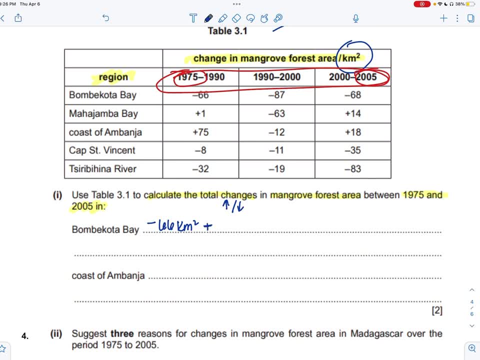 and then 1992 000 it and then 1992 000 it. lost another, lost another, lost another. so i guess i can add this, or so, yeah, so, yeah, so yeah, it lost another 87, it lost another 87. it lost another 87 because they want the total. so we're. 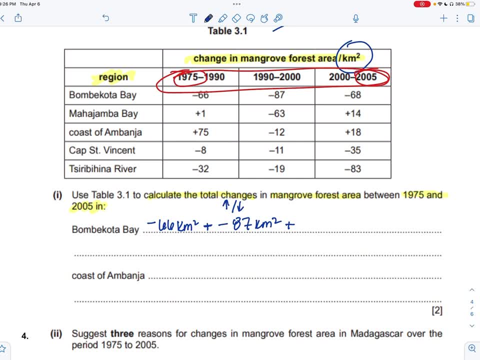 because they want the total, so we're. because they want the total, so we're going to put them together. going to put them together, going to put them together, and then, 2000 to 2005, they lost another, and then 2000 to 2005, they lost another. 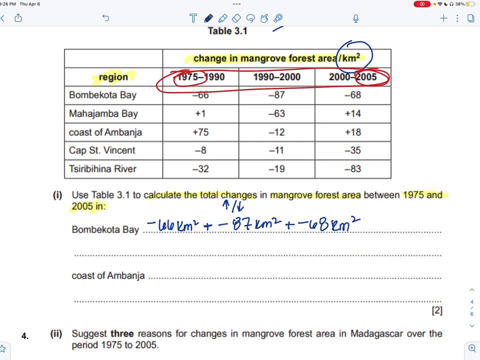 and then 2000 to 2005, they lost another 68.. i would do this on a calculator. i mean i would do this on a calculator. i mean i would do this on a calculator. i mean obviously, obviously, obviously. you know the kind of math i'm going to do. 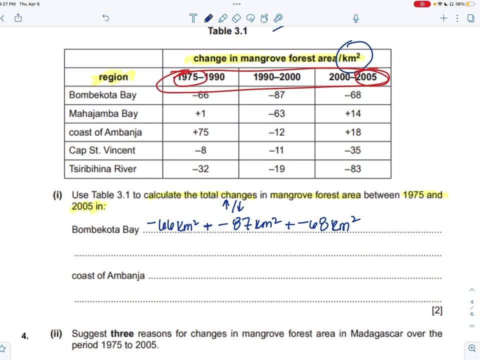 you know the kind of math i'm going to do. you know the kind of math i'm going to do, but the ipad doesn't have a calculator. but the ipad doesn't have a calculator. but the ipad doesn't have a calculator on it, like you have to download in. 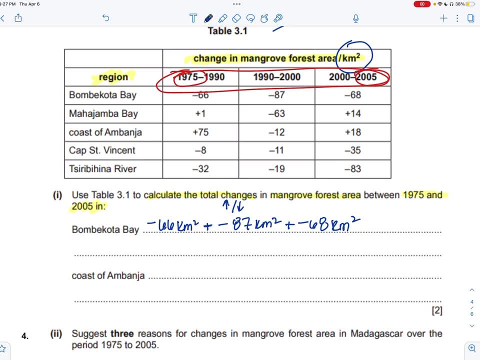 on it, like you have to download in on it, like you have to download in another app. which what a flaw. what a another app, which what a flaw, what a another app, which, what a flaw, what a flaw, flaw, flaw. but when you put these all together, do. 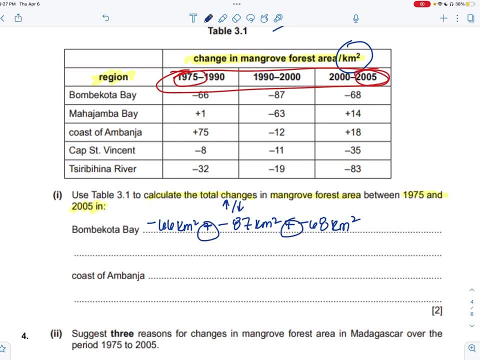 but when you put these all together, do, but when you put these all together, do your put togethers, your put togethers, your put togethers, you're adding them 66, 87 and 68, and you're adding them 66, 87 and 68 and. 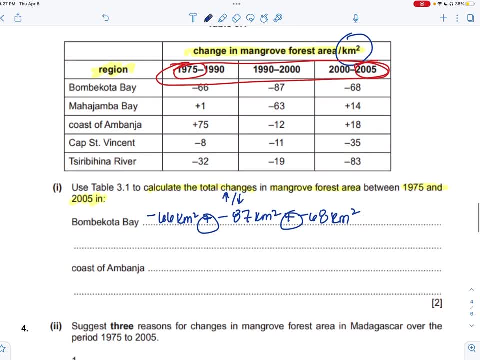 you're adding them 66, 87 and 68, and they're all negative. they're all losses. they're all negative. they're all losses. they're all negative, they're all losses. you're going to get a loss. you could say a decrease of 221 kilometers squared. 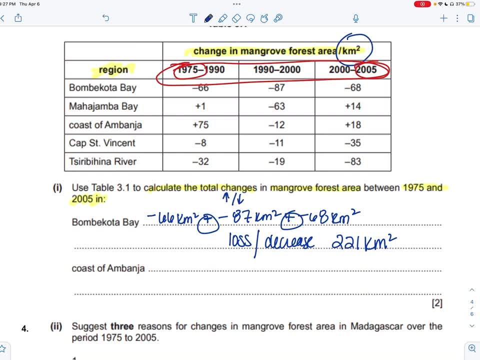 of 221 kilometers, squared of 221 kilometers, squared square kilometers. of 221 kilometers, squared square kilometers. please remember a unit or this. please remember a unit or this. please remember a unit or this, answer won't matter. and then answer won't matter. and then answer won't matter. and then ambanja and banja just kidding. 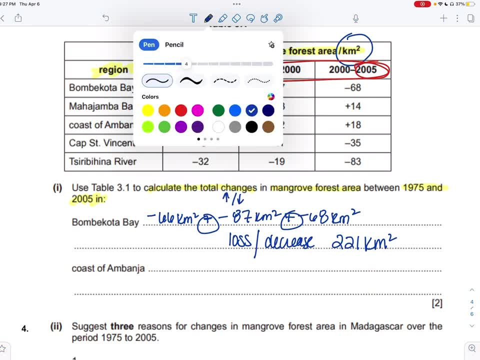 ambanja and banja just kidding ambanja and banja just kidding ambanja, maybe okay. so right here, 1975-1990, there was a okay. so right here, 1975-1990, there was a okay. so right here, 1975-1990, there was a gain of. 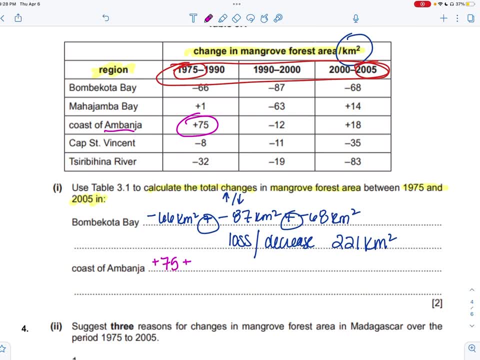 gain, of gain of 75, so a positive 75. if i want the 75, so a positive 75. if i want the 75, so a positive 75. if i want the total, so i'm going to total, so i'm going to total, so i'm going to add, and then 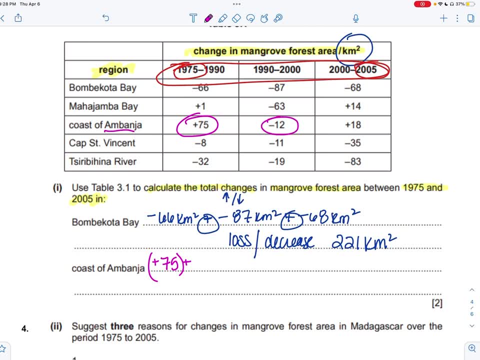 add, and then add, and then in that, in that, in that 10-year period 1992 000, 10-year period 1992 000, 10-year period 1992 000, they lost 12. and then in that five-year period 2005. 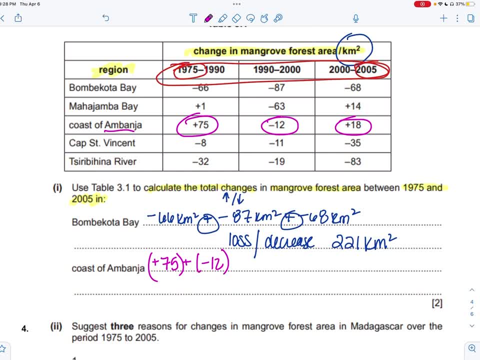 and then in that five-year period 2005, and then in that five-year period 2005, they gained another 18.. they gained another 18.. they gained another 18.. and they probably gaining another 18, and they probably gaining another 18. 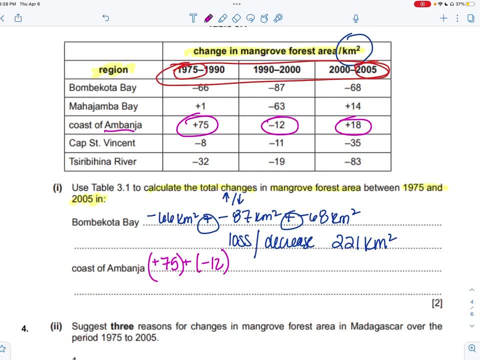 and they probably gaining another 18, which is based off one of like the last, which is based off one of like the last, which is based off one of like the last slide of notes, that last topic that you slide of notes, that last topic that you slide of notes, that last topic that you had about. 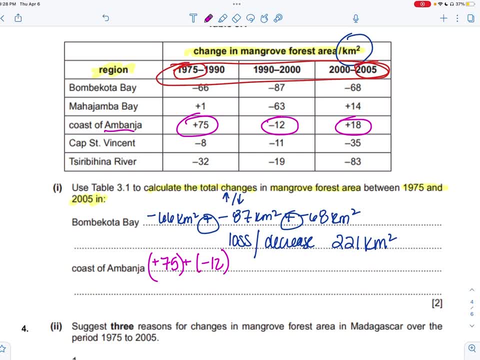 had about had about um human threats to the ecosystem, to um human threats to the ecosystem, to um human threats to the ecosystem to the mangrove forest, the mangrove forest, the mangrove forest, and that we were changing, it changing and that we were changing it changing. 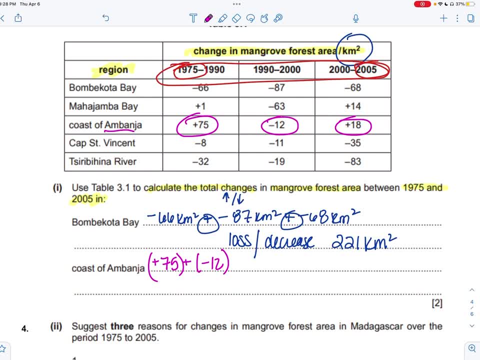 and that we were changing it, changing the land use for the land use, for the land use for infrastructure. so roads um infrastructure, so roads um infrastructure. so roads um streets, which i guess is the same thing, streets, which i guess is the same thing, streets, which i guess is the same thing as roads. 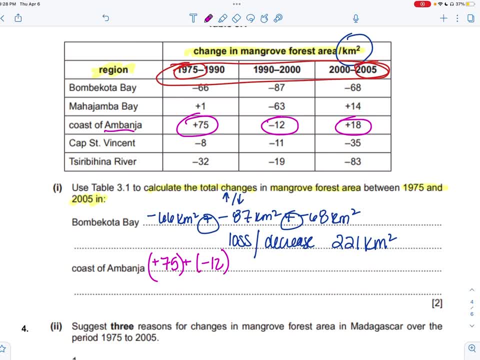 as roads, as roads. thank you so much. changing it to have shrimp farms, changing it to have shrimp farms, changing it to have shrimp farms, changing it to put like, changing it to put like, changing it to put like: golf courses, gosh, golf courses is, golf courses, gosh, golf courses is. 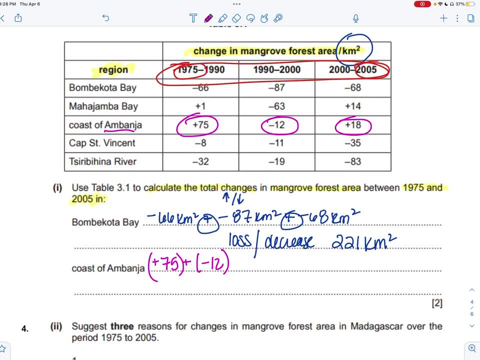 golf courses- gosh golf courses- is the bane of the environment. it is the the bane of the environment. it is the the bane of the environment. it is the worst, worst, worst. people are now trying to use wastewater. people are now trying to use wastewater. 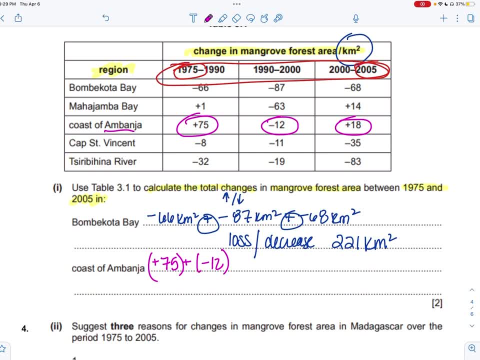 people are now trying to use wastewater- not black water but gray water, not black water but gray water, not black water but gray water- for watering golf courses, but it is just for watering golf courses, but it is just for watering golf courses, but it is just such a massive waste of resources. 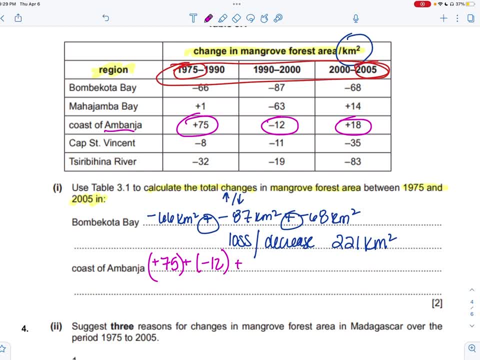 such a massive waste of resources. such a massive waste of resources. anyway, i'm assuming that that plus 18 is from. i'm assuming that that plus 18 is from. i'm assuming that that plus 18 is from mangrove restoration. that's all i was. 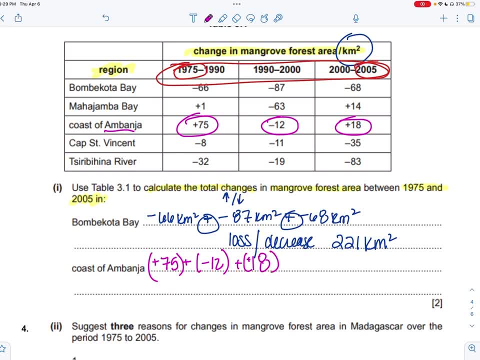 mangrove restoration. that's all i was. mangrove restoration, that's all i was trying to get at, trying to get at, trying to get at the replanting them. so did an increase of 75, then they lost 12. did an increase of 75, then they lost 12. 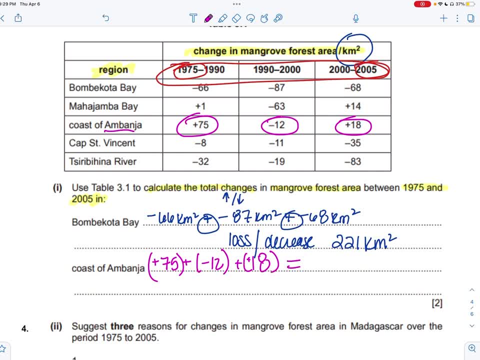 did an increase of 75, then they lost 12, and then another increase of 18, and then another increase of 18, and then another increase of 18. it's going to be, it's going to be, it's going to be a gain, a gain. 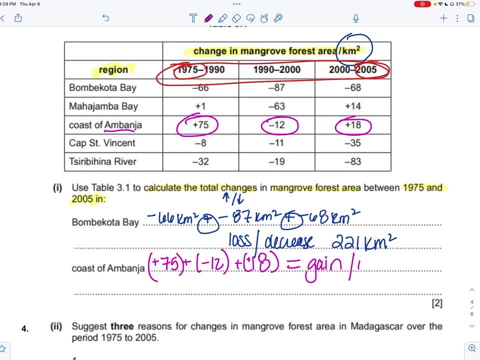 a gain just if you add those all together, just if you add those all together, just if you add those all together. remember it's negative. 12, though again. remember it's negative 12, though again. remember it's negative, 12, though again. or you could say an increase. 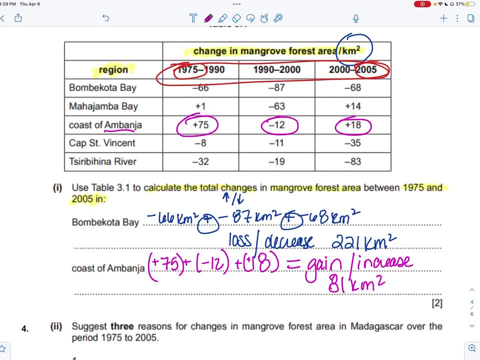 of 81 square kilometers again. don't of 81 square kilometers again. don't of 81 square kilometers again. don't forget the unit. forget the unit. forget the unit, otherwise it won't matter. i don't think. otherwise it won't matter, i don't think. 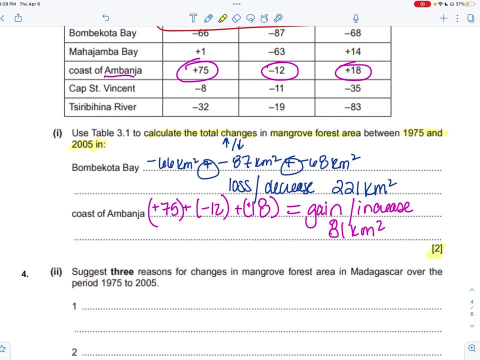 otherwise it won't matter. i don't think they would give. they would give, they would give partial credit on this, because it's partial credit on this, because it's partial credit on this, because it's only one market piece. so just three reasons for the change in. so just three reasons for the change in. so just three reasons for the change in mangrove forest: mangrove forest- mangrove forest- area in madagascar over the period 1975. area in madagascar over the period 1975. area in madagascar over the period 1975- 2005.. 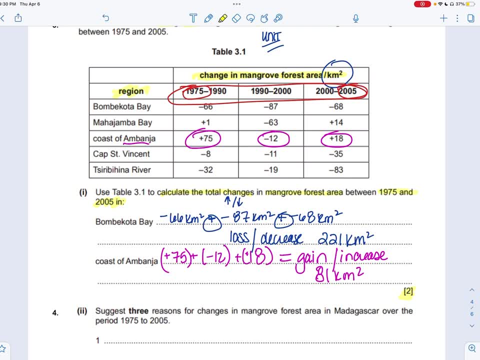 and this could be any of those regions, and this could be any of those regions and this could be any of those regions, any of them. so over here, we're going to any of them. so over here, we're going to any of them. so over here, we're going to have overall: 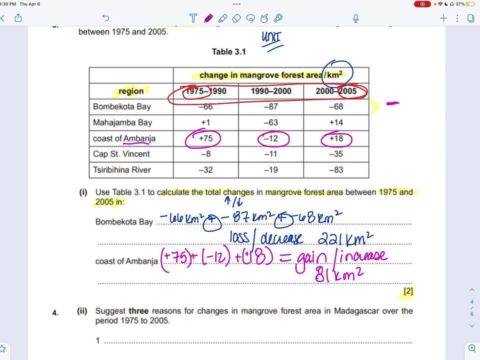 have overall. have overall um a loss. this is going to be a loss. um a loss. this is going to be a loss, um a loss. this is going to be a loss. mahajamba bay overall. mahajamba bay overall. mahajamba bay overall, even though they did have an increase. 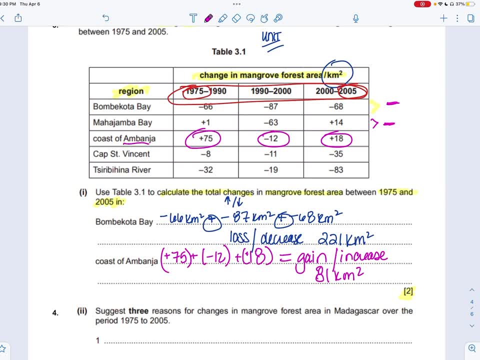 even though they did have an increase, even though they did have an increase from 2005 overall, there's still going to from 2005 overall. there's still going to from 2005 overall. there's still going to be a loss. ambanja, we saw there was a gain. 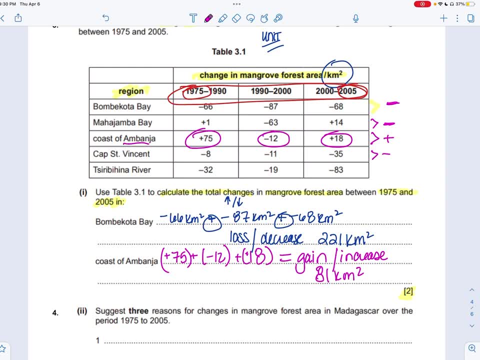 ambanja, we saw there was a gain. ambanja, we saw there was a gain. negative, negative, negative. there's going negative, negative, negative, there's going negative, negative, negative. there's going to be a loss to be a loss to be a loss. negative 32, negative, negative, definitely a. 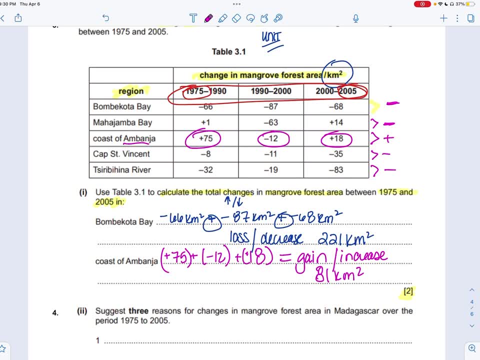 negative. 32 negative negative. definitely a negative. 32 negative negative: definitely a loss. i'm glad this wasn't one that i had to. i'm glad this wasn't one that i had to. i'm glad this wasn't one that i had to say out loud. 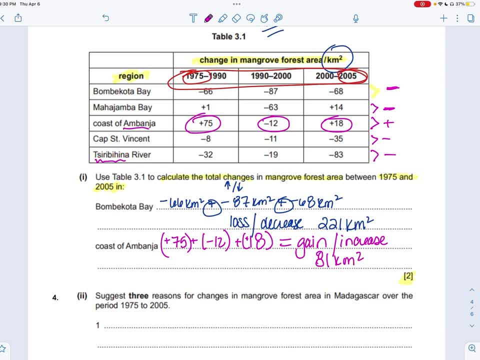 say out loud, say out loud, okay. so we can talk about reasons for okay. so we can talk about reasons for okay. so we can talk about reasons for the change. but we the change, but we the change, but we something that to notice, we can also, something that to notice, we can also 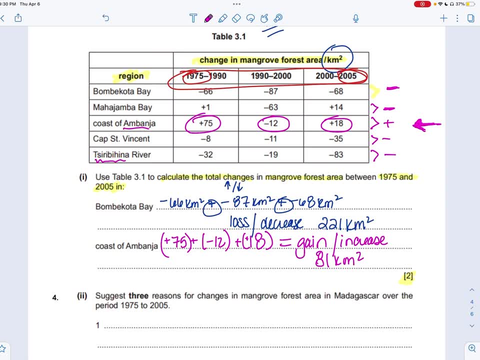 something that, to notice, we can also mention, mention, mention why there could possibly be a gain because of the ambanja coast. suggests because of the ambanja coast. suggests because of the ambanja coast. suggests three reasons, three reasons, three reasons for change in the mango forest between 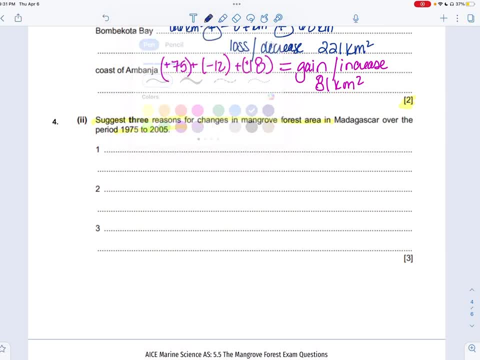 for change in the mango forest between: for change in the mango forest between 75 to 2000, 75 to 2000, 75 to 2000. okay, and this actually is very well supported and this actually is very well supported and this actually is very well supported in your notes. 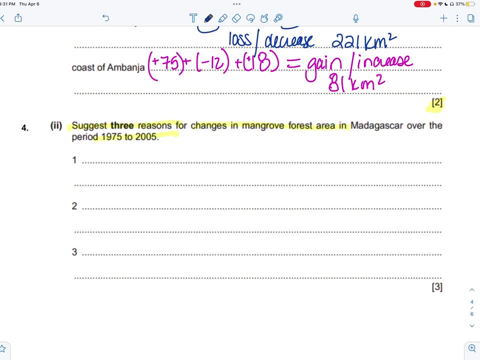 in your notes. in your notes, this question is also from paper 11 2022. this question is also from paper 11 2022. this question is also from paper 11 2022, may june, may june, may june. so specific, specific. 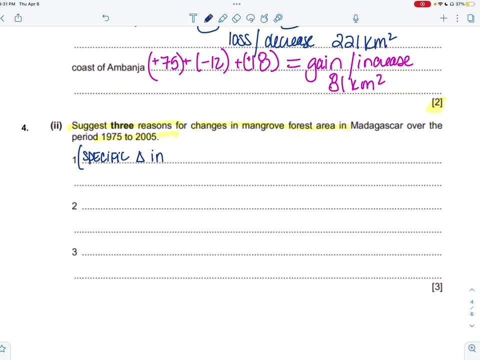 specific. specific: mention of a change, delta change. mention of a change, delta change. mention of a change, delta change in land use: that's not an answer. just that is the that's not an answer. just that is the. that's not an answer. just that is the guidance. you can't just say a change in. 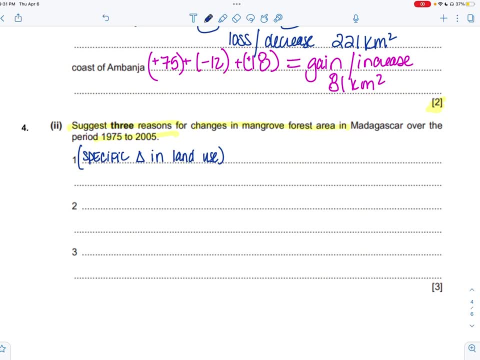 guidance. you can't just say a change in guidance. you can't just say a change in land use like what's the reason for the land use, like what's the reason for the land use, like what's the reason for the change in land use- shrimp farming. 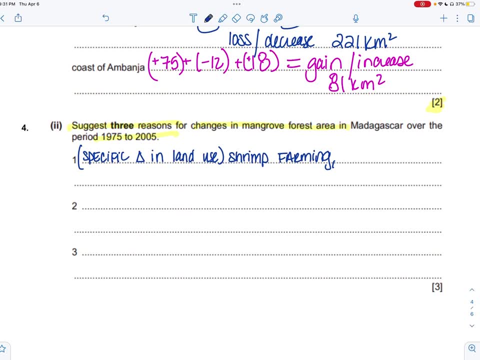 shrimp farming and they're realizing now, with the loss, and they're realizing now with the loss, and they're realizing now, with the loss of land from erosion, that shrimp farming of land from erosion, that shrimp farming of land from erosion, that shrimp farming wasn't ever going to net them more money. 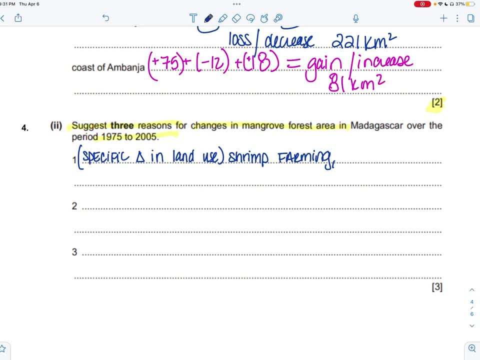 wasn't ever going to net them more money, wasn't ever going to net them more money than what they're losing, than what they're losing, than what they're losing due to coastal erosion, due to coastal erosion, due to coastal erosion, losing houses, losing houses, losing houses, tourism. 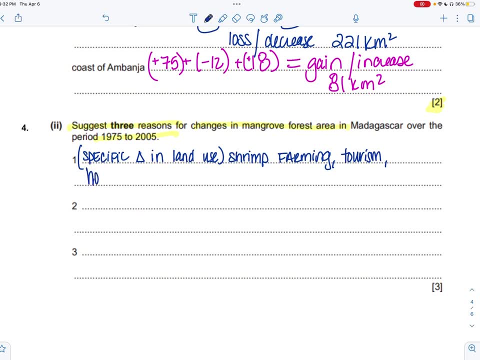 building resorts, building resorts, building resorts, housing, all within these same housing, all within these same housing, all within these same changing in land use, changing in land use, changing in land use, infrastructure, infrastructure, infrastructure, so transportation ways, um anything that's under the water, or um anything that's under the water, or? 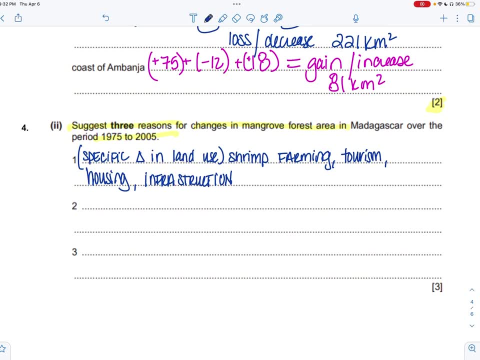 um, anything that's under the water or anything that's under the ground, anything that's under the ground, anything that's under the ground, electrical wires, pipes, water pipes, electrical wires, pipes, water pipes, electrical wires, pipes, water pipes, sidewalks, sidewalks, sidewalks, roads, things like that. all right, that'll be the first mark. 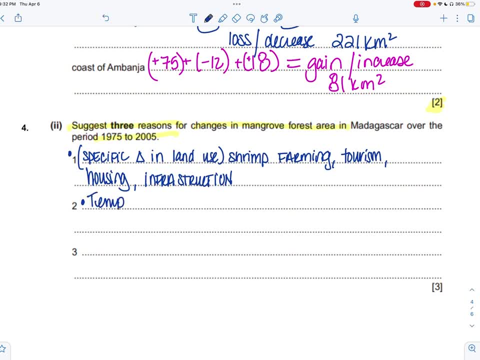 all right, that'll be the first mark. all right, that'll be the first mark we get to talk about in terms of what we get to talk about, in terms of what we get to talk about in terms of what the climate's doing. so, the climate's doing so. 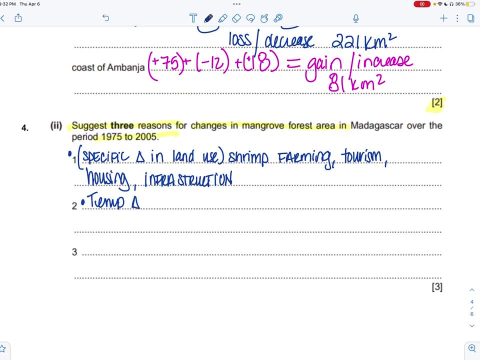 the climate's doing so. temperature changes, delta. temperature changes, delta. temperature changes: delta is a change in. i usually just use. is a change in. i usually just use. is a change in. i usually just use that. it's just a quick symbol for doing that. it's just a quick symbol for doing. 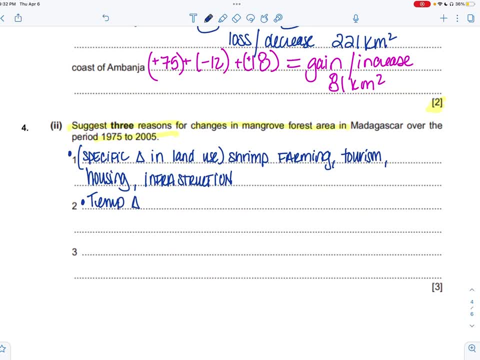 that it's just a quick symbol for doing things like this, things like this, things like this. please don't write that on your exam. climate change, global warming- you absolutely would not global warming. you absolutely would not. global warming. you absolutely would not want to put for number one. 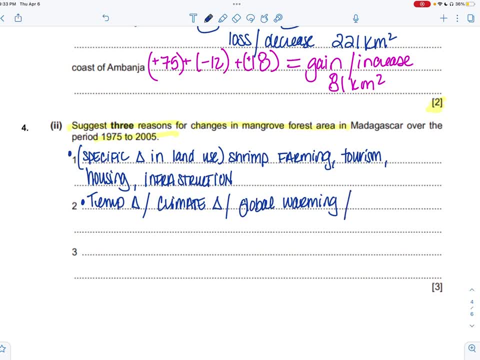 want to put for number one, want to put for number one: global warming, number two: climate change. global warming number two, climate change. global warming, number two: climate change. you're essentially, you're essentially, you're essentially saying the same thing: climate change. saying the same thing, climate change. 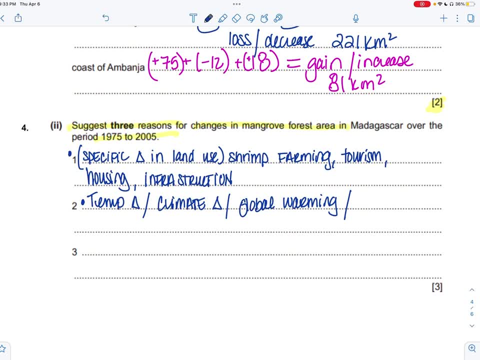 saying the same thing: climate change causes global warming, causes global warming, causes global warming um increase in sea level. all of these um increase in sea level. all of these um increase in sea level. all of these are part of the same, are part of the same, are part of the same idea. 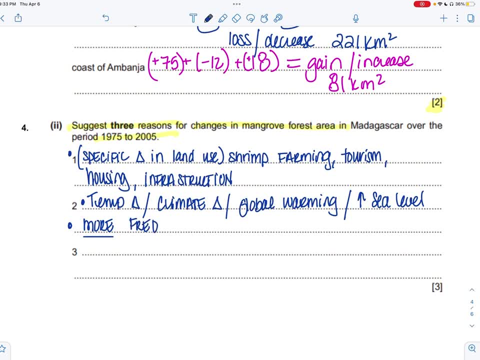 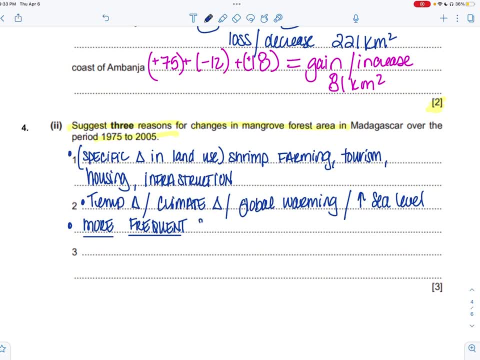 frequency. frequency, frequency, or increasing the rate of storms, or increasing the rate of storms, or increasing the rate of storms, could also say specific like hurricanes. could also say specific like hurricanes. could also say specific like hurricanes that definitely can damage our shorelines, that definitely can damage our shorelines. 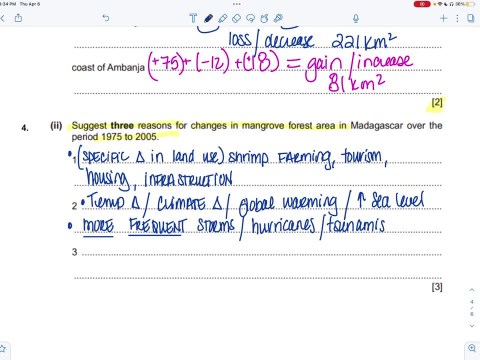 that definitely can damage our shorelines. my favorite: tsunamis, and, and, and. if you're watching this, maybe you're. if you're watching this, maybe you're. if you're watching this, maybe you're not in america. not in america. not in america or in north america. typhoons are also. 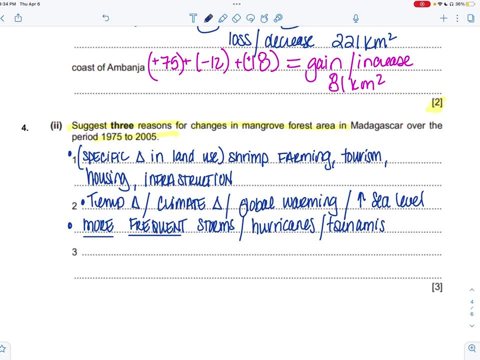 or in north america typhoons are also, or in north america, typhoons are also an answer, an answer, an answer: tropical cyclones, but we typically don't tropical cyclones, but we typically don't tropical cyclones, but we typically don't call them that here. 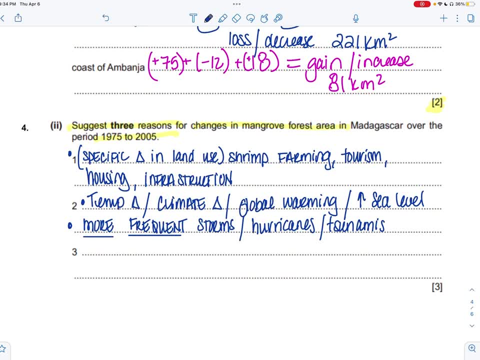 call them that here. call them that here. we just call them hurricanes. all right, um, all right, um. all right. um another one over harvesting timber. this also could be just chalked down to this also could be just chalked down to. this also could be just chalked down to deforestation. 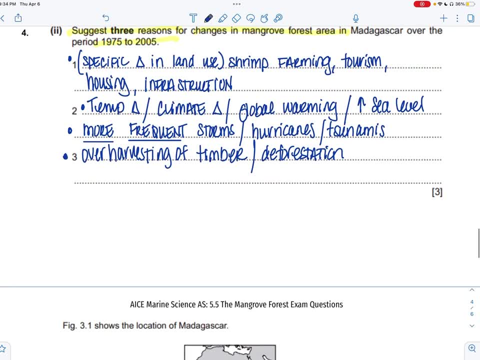 deforestation, deforestation. my favorite cop-out answer is what i? my favorite cop-out answer is what i? my favorite cop-out answer is what. i refer to it because, if you're talking, refer to it. because, if you're talking, refer to it because if you're talking about a decrease in population, 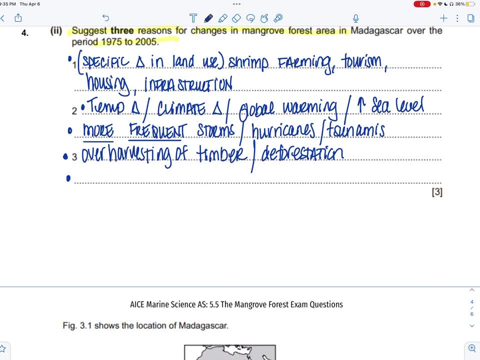 about a decrease in population, about a decrease in population. um, sorry for them, um, sorry for them, um, sorry for them. an easy answer that we can write. and it an easy answer that we can write. and it an easy answer that we can write. and it goes a lot of the time for a decrease. 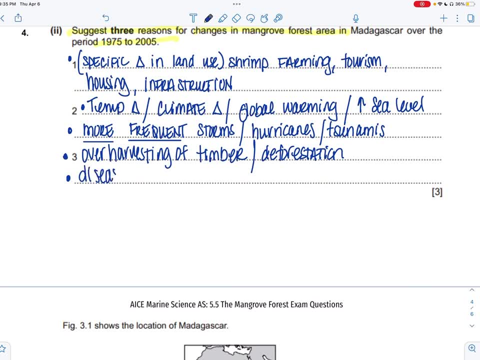 goes a lot of the time for a decrease, goes a lot of the time for a decrease in population, in population, in population disease. disease is definitely more frequent too. disease is definitely more frequent too. disease is definitely more frequent too whenever you have an increase in, whenever you have an increase in. 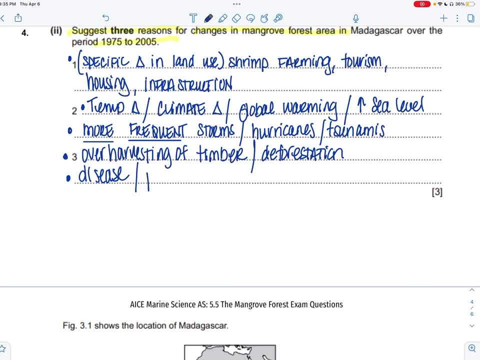 whenever you have an increase in temperature, they just spread more temperature, they just spread more temperature, they just spread more. also within this mark, if you mentioned also within this mark, if you mentioned also within this mark, if you mentioned parasites, but honestly i wouldn't think parasites, but honestly i wouldn't think. 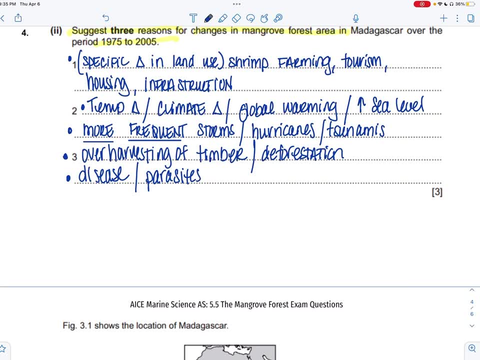 parasites. but honestly, i wouldn't think to write that because i i really wouldn't to write that, because i i really wouldn't to write that, because i i really wouldn't always be associating plants with always be associating plants with always be associating plants with parasites, though i know they can get. 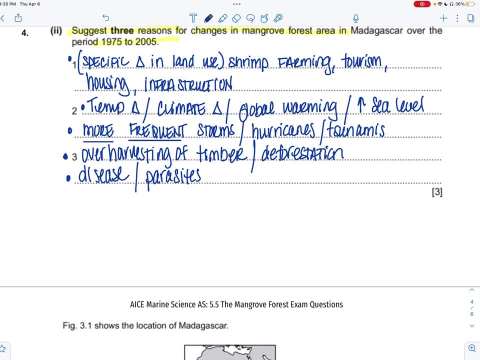 parasites, though i know they can get parasites, though i know they can get them, it just wouldn't have been my main them, it just wouldn't have been my main them, it just wouldn't have been my main go-to cause, go-to cause, go-to cause. and then, if we are considering the 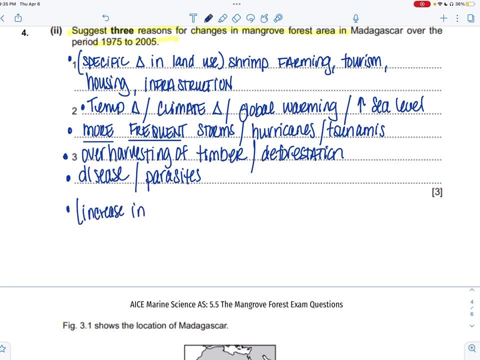 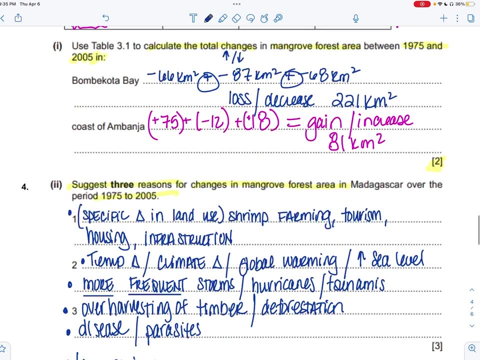 and then, if we are considering the, and then, if we are considering the increase, an area, and that one's from the an area, and that one's from the an area and that one's from the ambanja coast of ambanja, ambanja coast of ambanja. 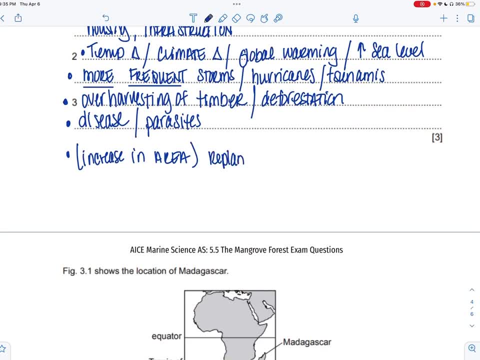 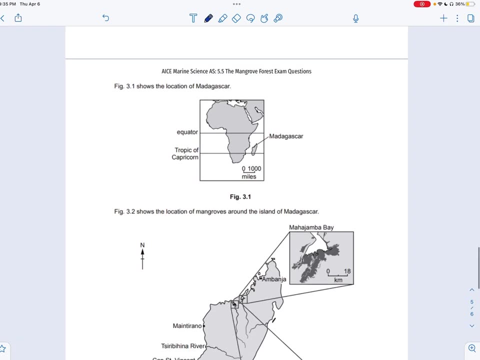 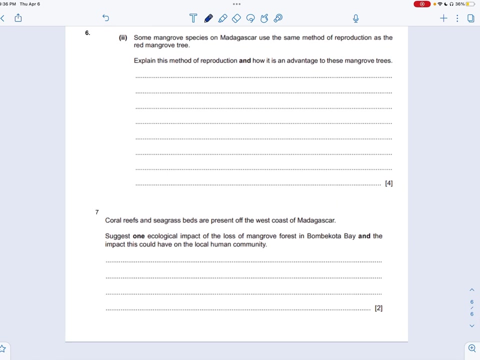 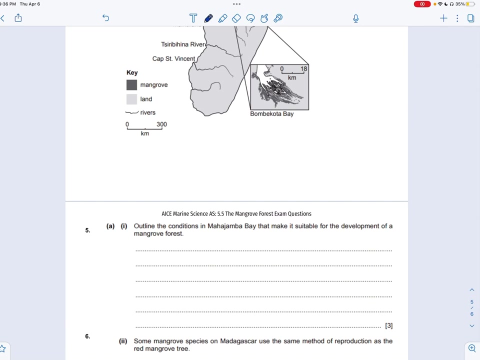 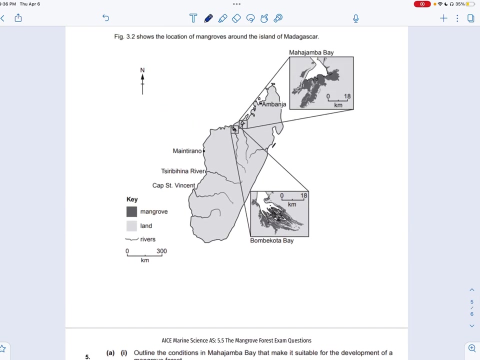 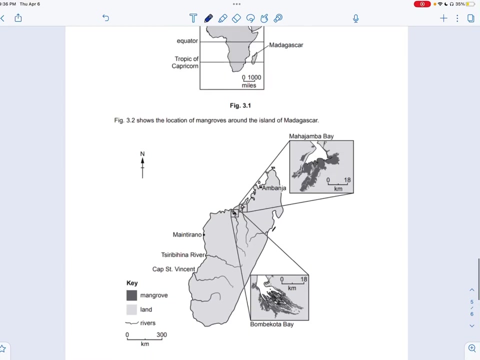 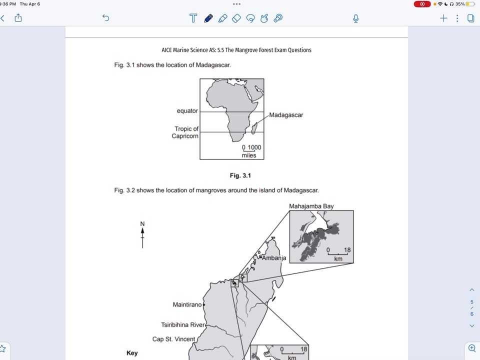 ambanja, coast of ambanja. a cause for that would be replanting of mangroves. okay, It's also a repeated topic in a level. it's also a repeated topic in a level. it's also a repeated topic in a level. so, looking at madagascar, 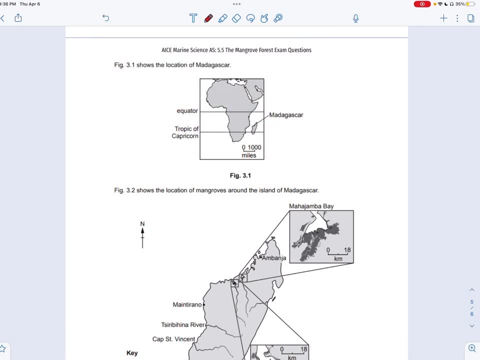 so looking at madagascar, so looking at madagascar, right away, something that i noticed, and right away something that i noticed, and right away something that i noticed, and just from doing these a lot, just from doing these a lot, just from doing these a lot, they're showing you a map. 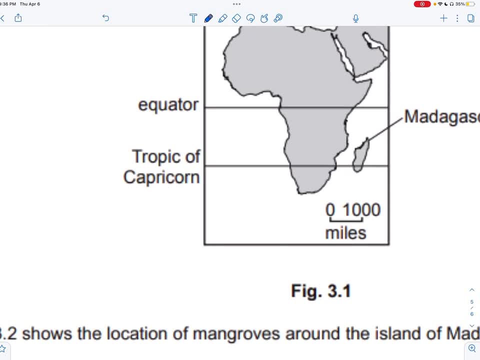 they're showing you a map. they're showing you a map, they show you the equator. they show you the equator, they show you the equator and they're showing you the tropic of and they're showing you the tropic of and they're showing you the tropic of capricorn. 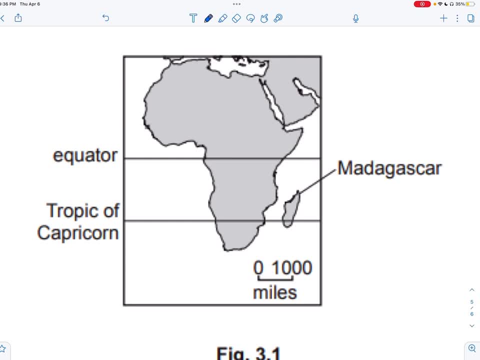 capricorn. capricorn, i bet you're going to need to reference. i bet you're going to need to reference. i bet you're going to need to reference it, or you can reference it, it, or you can reference it, it or you can reference it. sometimes the question says: and without? 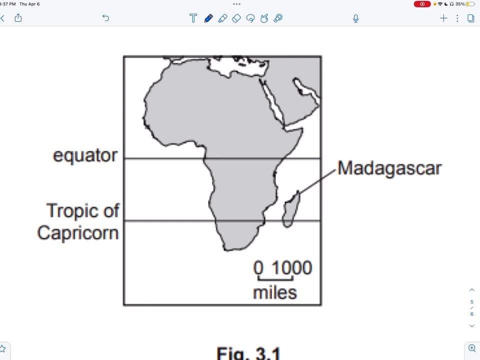 sometimes the question says: and without. sometimes the question says: and without even looking at it, even looking at it, even looking at it: um, sometimes the question says um. sometimes the question says um. sometimes the question says: using figure 3.1, using figure 3.1. 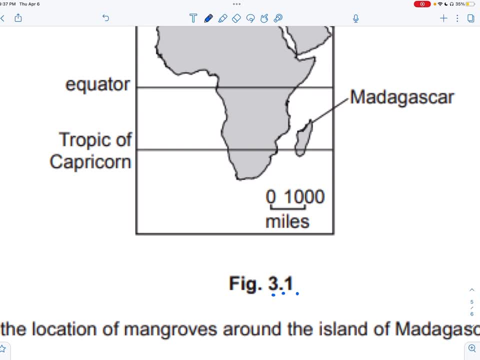 using figure 3.1, which is what you have here, though that, which is what you have here, though that, which is what you have here, though that it's not going to say that, it's not going to say that, it's not going to say that, but this, this is like the kinds of but this, this is like the kinds of, but this, this is like the kinds of things. they want you to reference things. they want you to reference things they want you to reference. it's a good hint that if they're, it's a good hint that if they're. 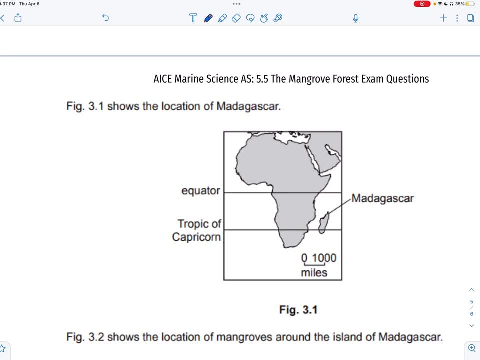 it's a good hint that if they're showing you a map, showing you a map, showing you a map, they want you to maybe reference the map. they want you to maybe reference the map. they want you to maybe reference the map anyway, anyway. anyway, the equator is zero degrees. 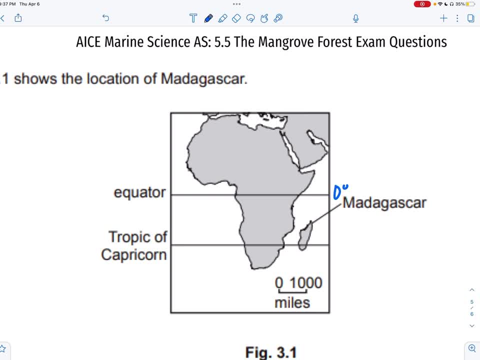 the equator is zero degrees. the equator is zero degrees. tropic of capricorn, tropic of capricorn. tropic of capricorn. the opposite of it is the tropic of the opposite of it is the tropic of the opposite of it is the tropic of cancer, and that is. 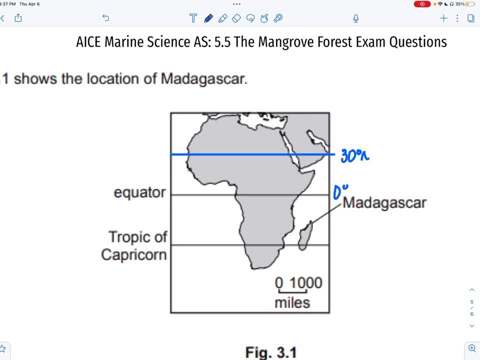 cancer and that is cancer and that is above the equator. specifically, it's 30 above the equator. specifically, it's 30 above the equator. specifically, it's 30 degrees north of the equator, though it's degrees north of the equator, though it's. 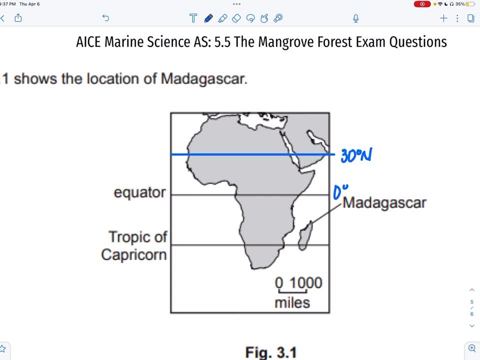 degrees north of the equator, though it's not put on there, not put on there, not put on there, just comparing it to us in the northern, just comparing it to us in the northern, just comparing it to us in the northern hemisphere, hemisphere, hemisphere, tropic of capricorn is 30 degrees south. 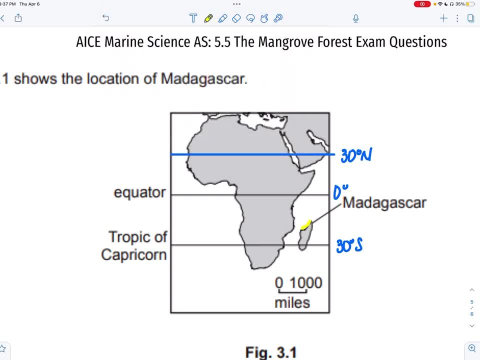 tropic of capricorn is 30 degrees south, tropic of capricorn is 30 degrees south, and if we see sweet little madagascar, and if we see sweet little madagascar, and if we see sweet little madagascar, she is right above it. 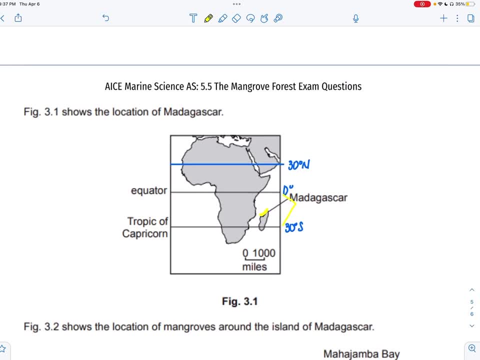 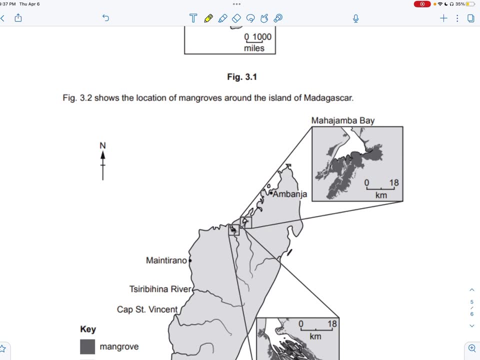 so, within this area, all right. so we're looking at the all right. so we're looking at the all right. so we're looking at the location of mangroves around the island, location of mangroves around the island, location of mangroves around the island of madagascar. so you have the whole. 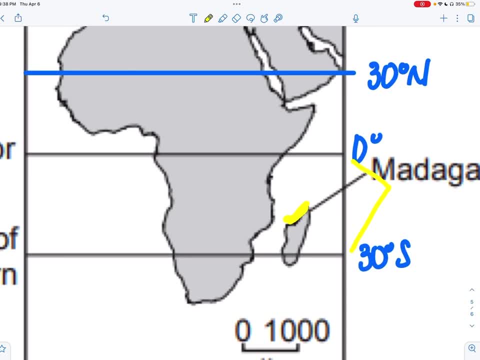 of madagascar. so you have the whole of madagascar, so you have the whole continent of africa here, and then you continent of africa here, and then you continent of africa here, and then you have just madagascar down here in the, have just madagascar down here in the. 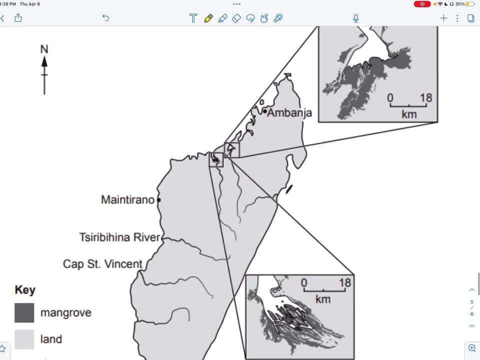 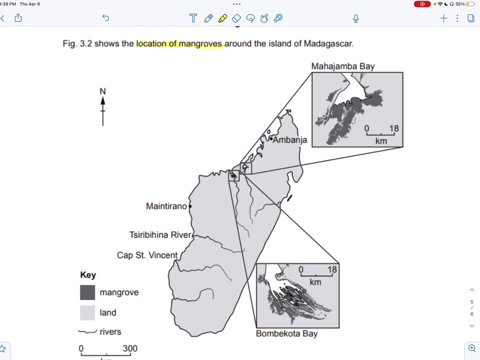 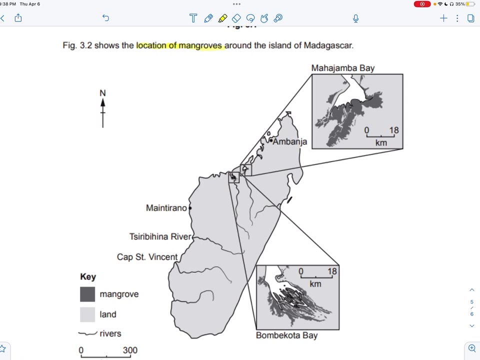 have just madagascar down here in the right, right, right, and then they're showing madagascar- i'm on the last questions and then even more zooming in. this top square is the mahajamba. this top square is the mahajamba. this top square is the mahajamba bay. i know in your paper you don't see. 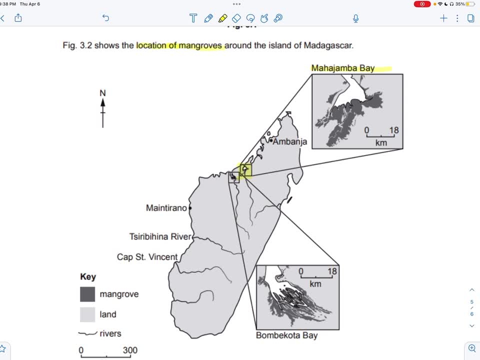 bay, i know in your paper you don't see bay, i know in your paper you don't see this as clear as me. but if you want this as clear as me, but if you want it printed out bigger, you do have. no, you don't. maybe you do, i can't remember. i'm going to check. 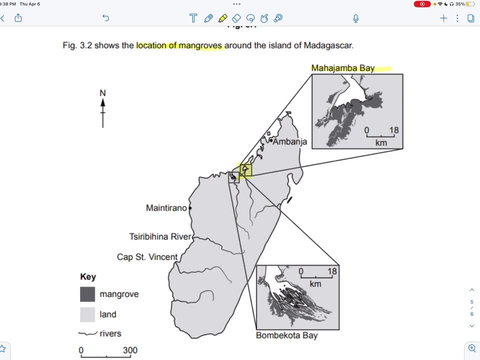 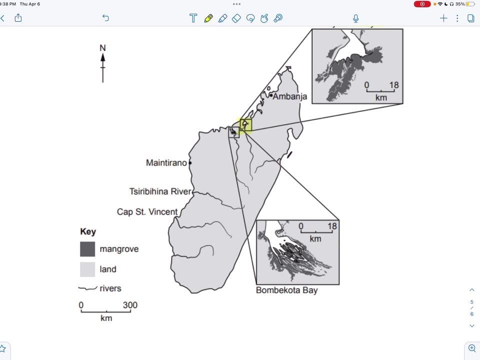 when this is over. i was going to say if you have the blank copies, you've got them in class, but if you want to see it bigger, you have it here or you can also print it out yourself. mahajama bay: looking at the key mangroves are the darker gray and i know it's not as easy to. 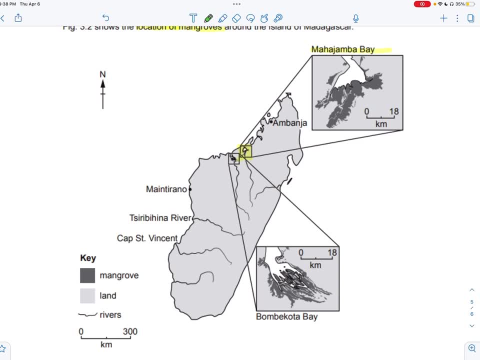 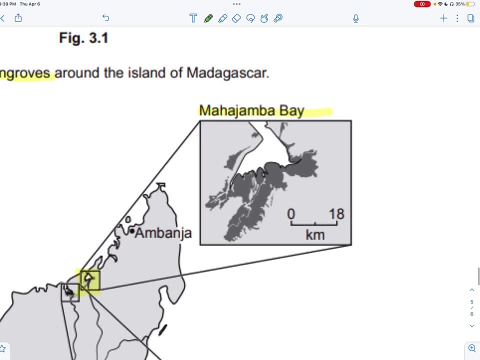 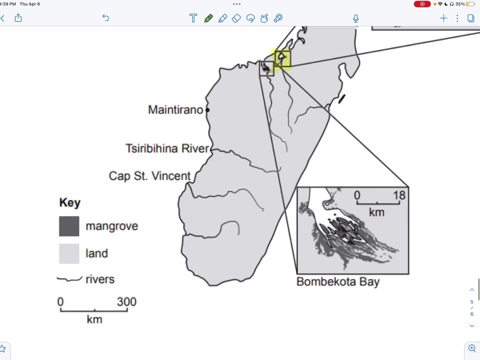 see on your paper, because i have the hash copies too. and then land, it's just your light gray rivers are the darker squiggles. so all this is mangrove, all the things that you see in the dark gray. okay, all this mangrove and then same down here. 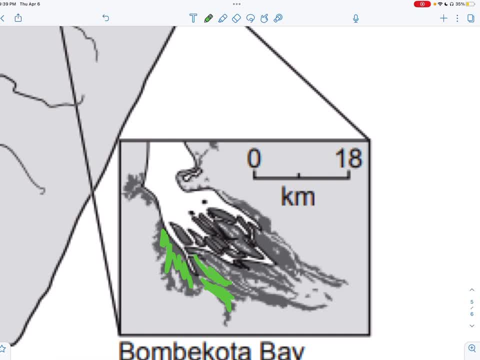 all mangrove everything in the dark gray. remember: you're allowed to use color on the exam, on questions, so you could definitely do something like this if that was better for you. i always recommend it. whenever there's maybe a graph with two different lines, you cannot use color on your. 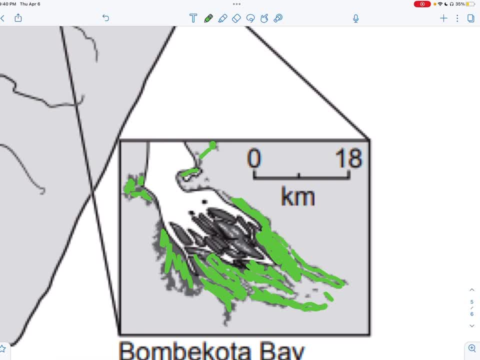 own answers, your own graph on your own answers. you can't use color on your own answers. your own graph on biological drawings you can. you can use it to color code the question, though you just can't use it for your answer. so take that as you like, okay, and all the little areas within here. 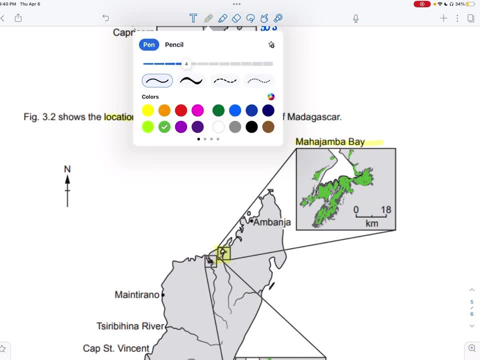 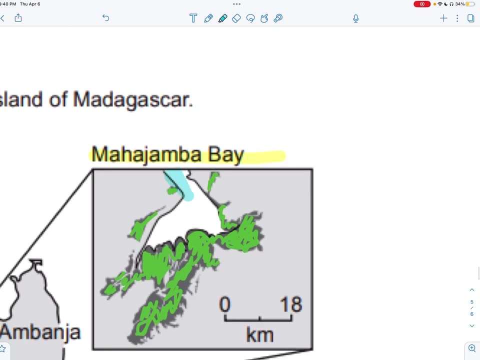 okay, yeah, and so the dark gray is land. so this is gonna be water. this part is water coming in, just so you can visualize it, and then all of this is going to be land. okay, there we go, and it's water coming in from the indian ocean. 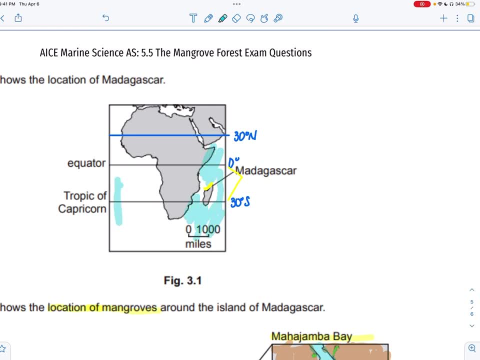 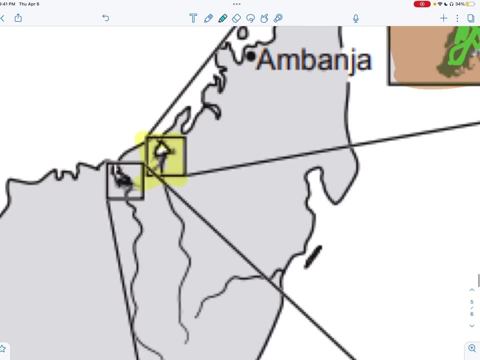 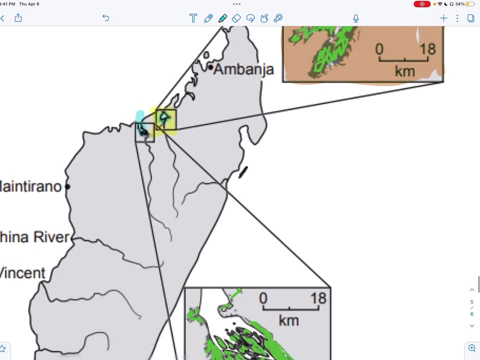 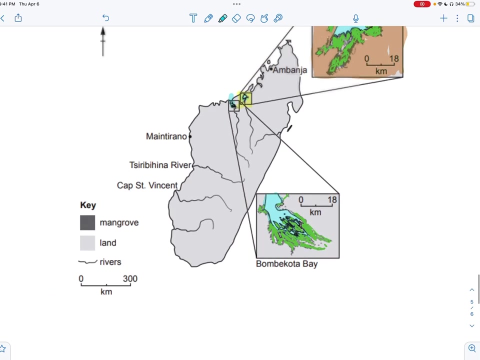 indian ocean is all over here. here's this side, it's the atlantic. you can see like the little indent here if i zoom in water and then same right here water. so this is from the indian ocean, definitely an estuarine area, and then rivers, the indian ocean. 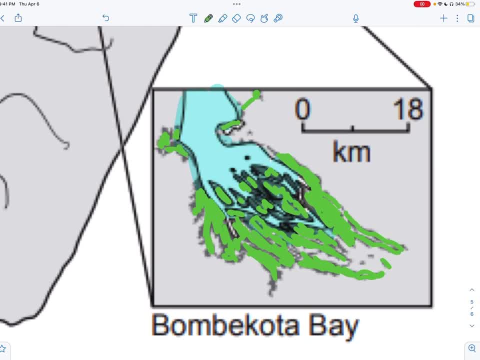 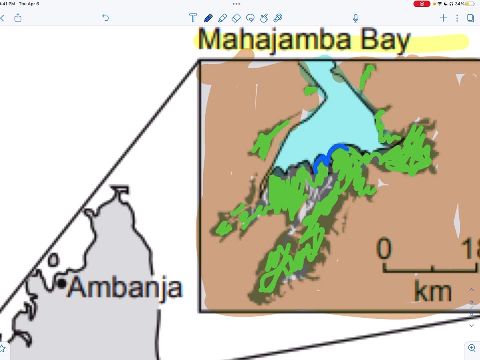 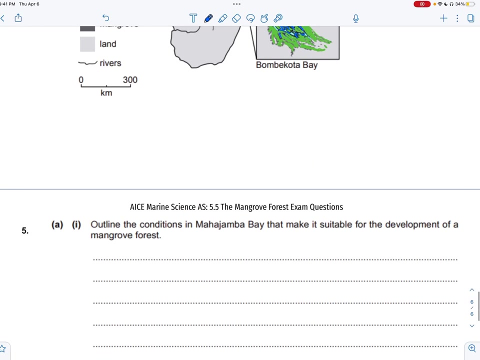 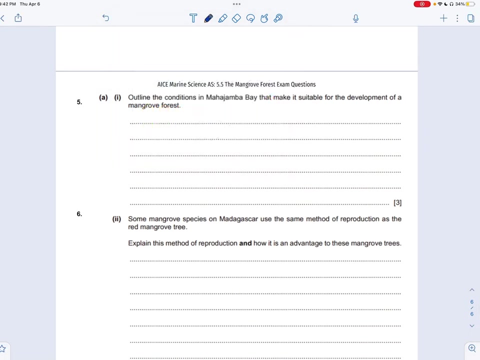 squiggle like lines. you can see. they're like the darker black lines on here, these, these black lines. so you have freshwater input water coming in from the ocean, definitely an estuary, so you brackish water. intercoastal areas- here's the river. okay, and all of that just for this question. outline the conditions in? 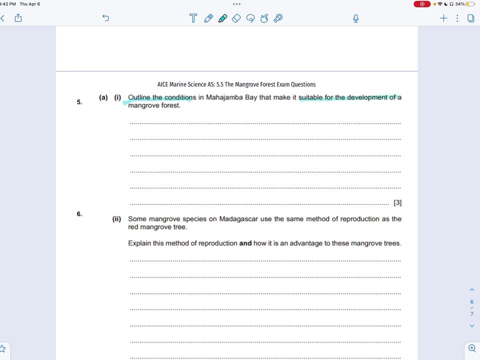 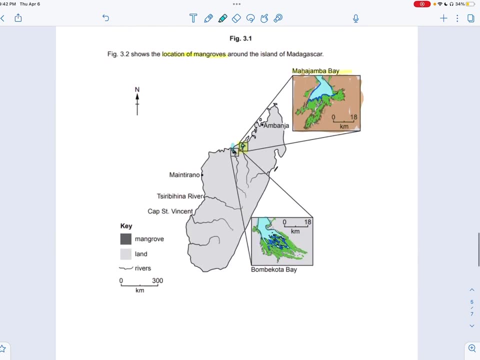 Mahashamba Bay that make it suitable for the development of a mangrove forest. so this is going to be like the first two boxes you guys filled in in your note page that was in the description box and then you're going to be able to see the 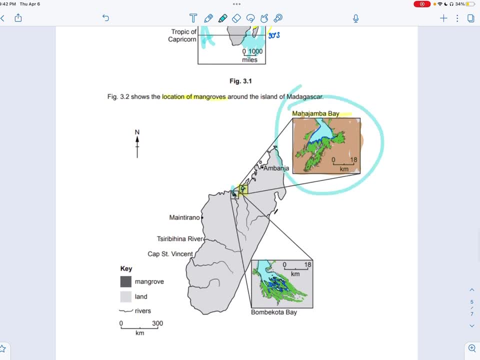 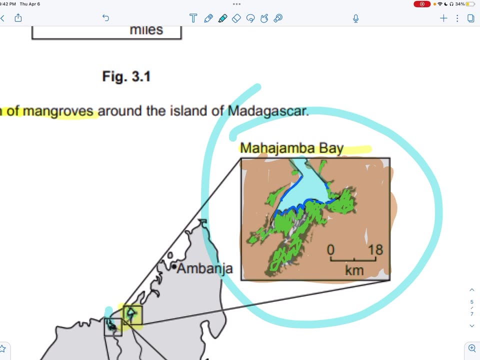 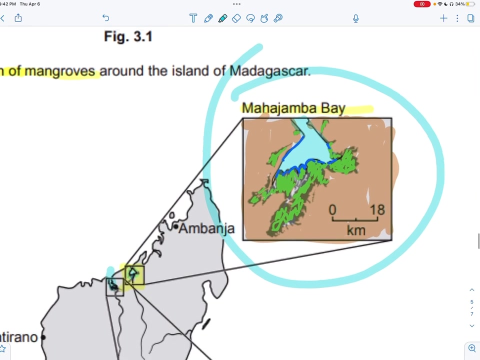 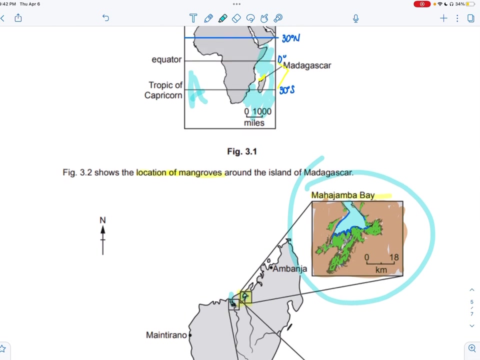 video I posted earlier. here's the Mahashamba Bay and so, like we I just covered, it is influenced by ocean, so saltwater. it has freshwater input from rivers. definitely we need to mention that it is in a subtropical or tropical climate. I'm sure the water will be shallow. it's going to be a little bit more shallow. 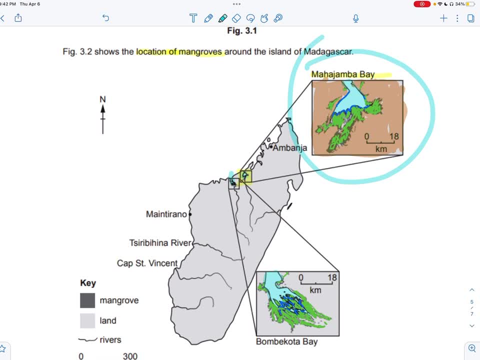 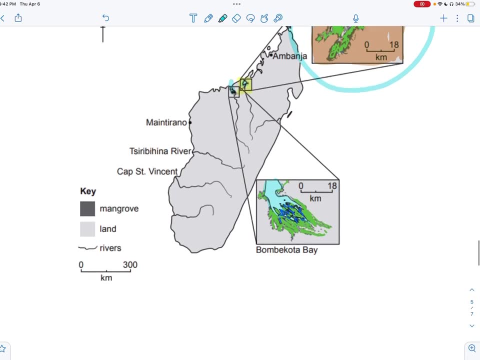 I'm sure the water will be shallow. it's going to be a little bit more shallow very close to land and if it's an estuary type area, that also needs to happen. estuaries are intertidal��도 talk about it being intertidal with a. 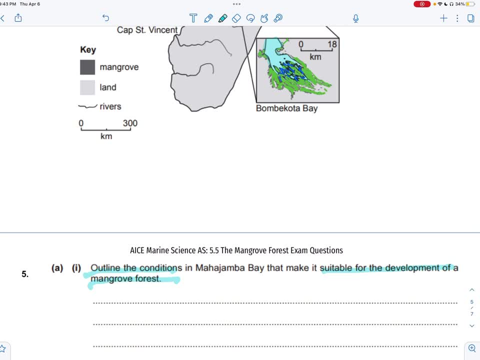 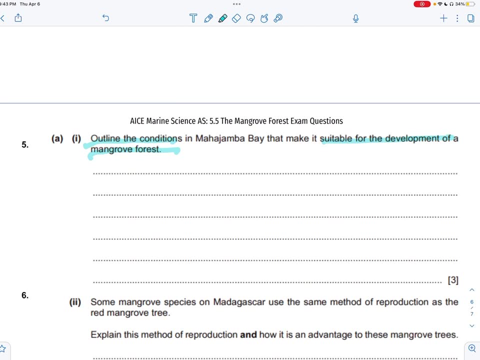 definition of an estuary is a partially enclosed tidal body of water. within those conditions, we also need to make sure that the water is relatively calm. it typically isn't an estuary, so you can have sedimentation of silt. if you look at your influence on tua and novipsuripura, which are the bases of saltwaterныshuru values, since the facility that you get very close to land, if it's an estuary type area, that also needs to happen. 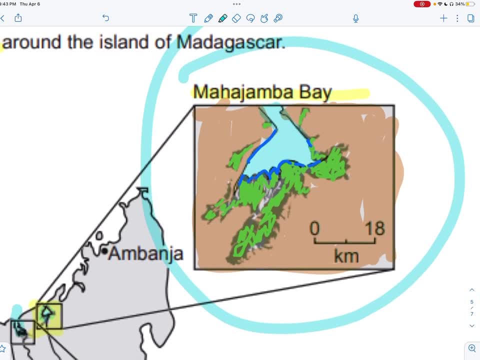 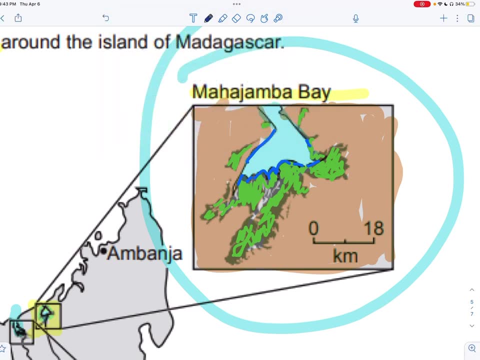 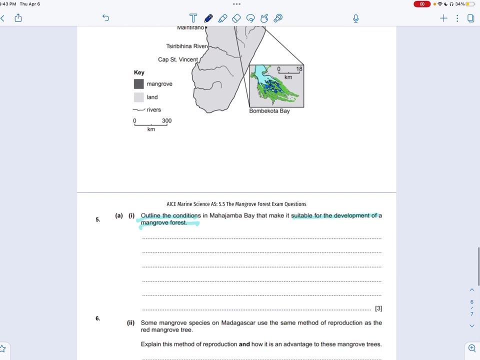 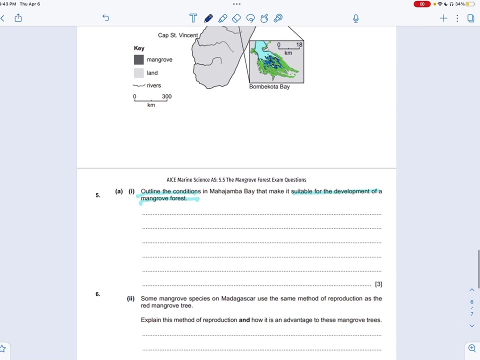 your influence to land this, all the ground areas. surely you're going to have some sediment runoff, or runoff that contains dissolved sediments in there, dissolved nutrients that can help with with the growth, protein production, dna production, what else? enzymes anyway, making chlorophyll okay. so just outline the conditions and it's three marks. we need at least three things. 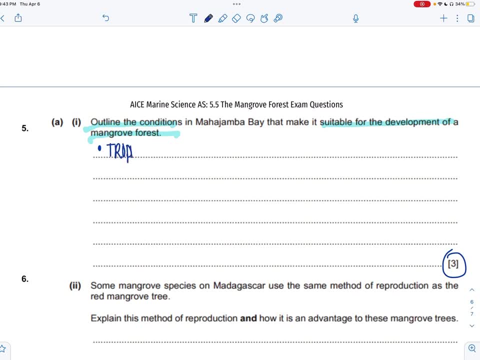 so they're in a tropical or they need subtropical climates. uh, you could also be specific and i shouldn't put a slash parentheses: 25 degrees north to 25 degrees south. so you could also be specific. so you could also be specific and i shouldn't put a slash parentheses: 25 degrees north to 25 degrees south. 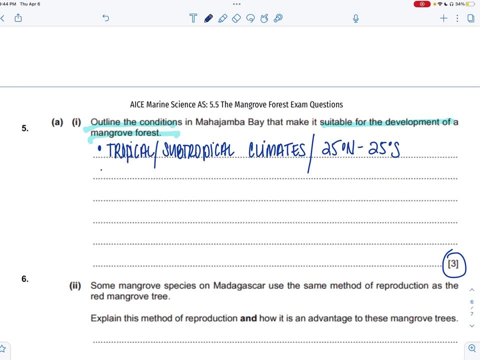 so you could also be specific and i shouldn't put a slash parentheses: 25 degrees north to 25 degrees south. it's an inter-tidal area so influenced by the tides, with saline water from the indian ocean to the into the earth, clandestine and fresh water. 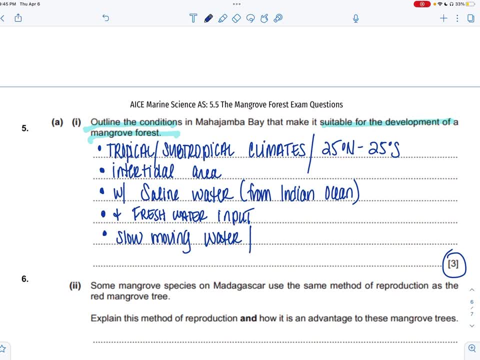 input. okay, low wave action, calm water, all that jazz being shallow, so something along those lines, so that we can mention this- will allow for sedimentation: the process of sediments being deposited, of fine sediments or fine grains. that gains grains and then one more sediment runoff. 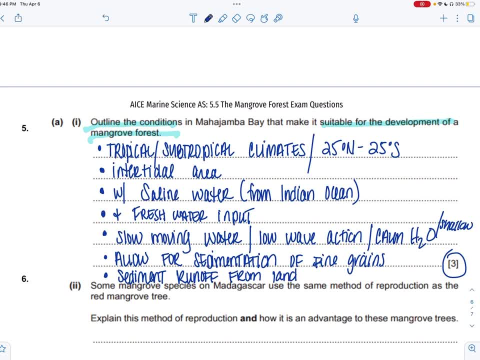 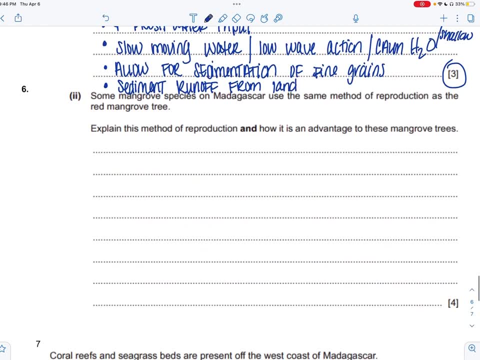 land maybe you could mention like runoff containing nutrients from land that will also help their growth. some mangrove species in Madagascar use the same method of reproduction as the red mangrove tree, and that is what is featured in your syllabus. it's also what is in the notes that you have. so some mangrove species Madagascar use the same method of. 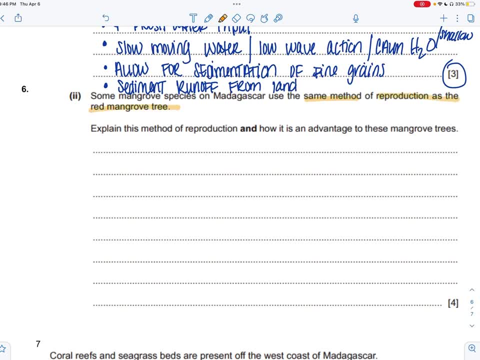 reproduction as the red mangrove tree. there's a lot of species of mangroves. Florida typically only has, I think, just three: red mangrove, black mangrove and a white mangrove. explain so, why and how this method of reproduction. so explain why and how it is an advantage to these mangrove trees. so explain the method of. 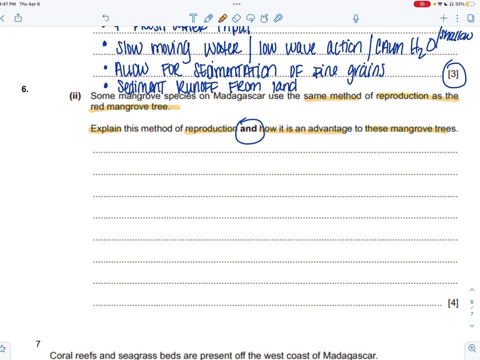 the reproduction method, which is vivibrous. and then, how is this an advantage to the mangrove tree? how does that method help them? and we only got one more question after this. okay, so we should definitely reference the method. mangroves are viviparous. 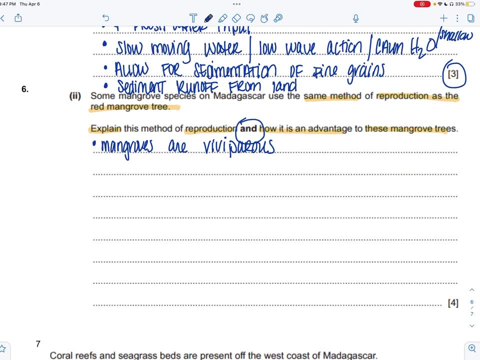 that v-i-v-i- the vivi is referring to it- living on the parent. for for a little bit, like I mentioned, it doesn't just drop the seed. the seed is going to grow into a propagule while still being attached, and we can write about that. the seeds remain. 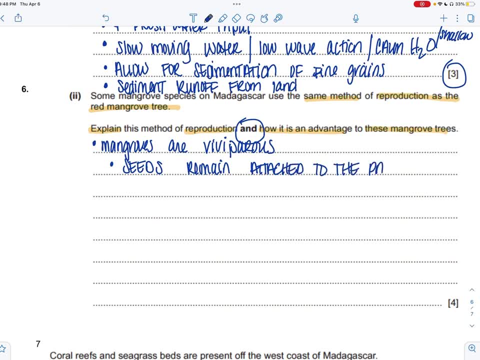 attached to the parent. and something you guys might be noticing is that there's some more detail in these exam answers than they have in the textbook, which sometimes is frustrating, like how could you expect somebody to be able to produce this on an exam answer if it wasn't an expectation in the main source of content? but this is why doing these are. 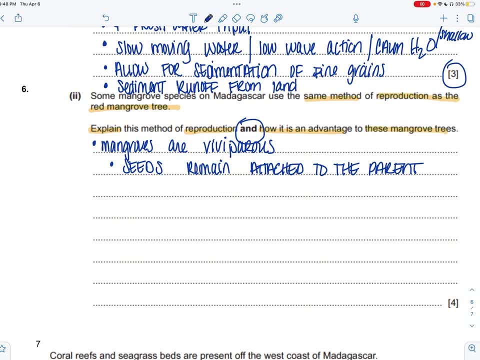 definitely an advantage. um and so like, explain, like why, would they say, on their parent plant, so the seeds could not survive in a saline environment? the propagules can, but the seeds can't, and so they- meaning the seeds- gain water and nutrients from the parent. something I wouldn't have thought to write, but again just repeat: this is why we do exam questions. 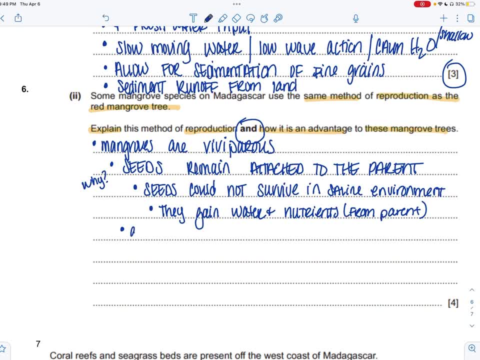 so while they're attached to the parent, germination occurs. so it's like when it actually emerges from its seed to start to germinate and start to grow, and while it's still attached to the parent. it's already mentioned so you don't need to really mention again while still attached. 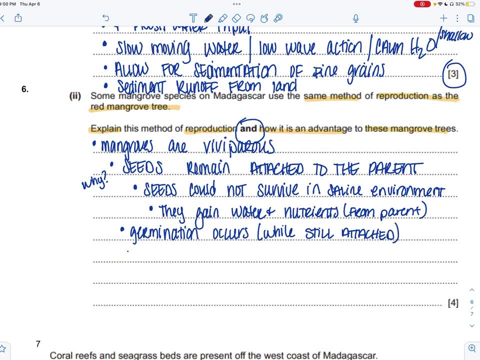 foreign. either button orkan button. our bedside wood, seminoles and peottus magnificium carotene and other people at different locations, people sitting in a big plot yard or say middle of the WOI, biraz last night, we color your seeds. I'd like to see tall trouts. 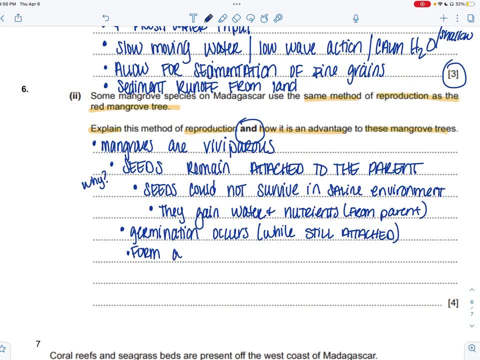 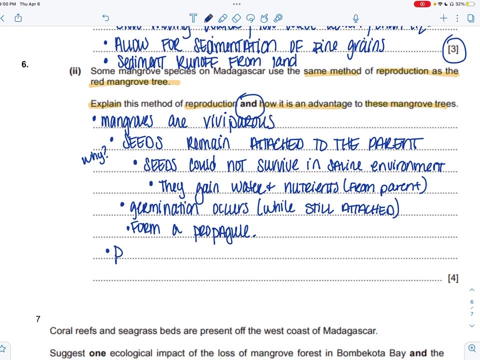 and this will form a propagule and it's not until it's a propagule that it gets dropped. the propagule will drop into the ocean water or drops into the ocean or floats an ocean. at this point it can survive. this is that elongated structure with smaller, little prop roots going and they'll have like. 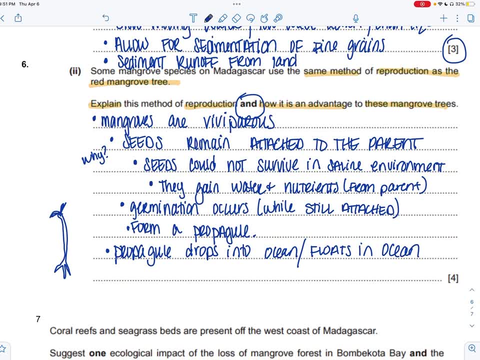 their leaves starting to grow at the top. they really won't start growing their leaves until they can embed themselves in some sediment when they find a very soft sandy substrate. sometimes you see them hanging off mangroves and they have some of those root structures already growing, the little propagules anyway. 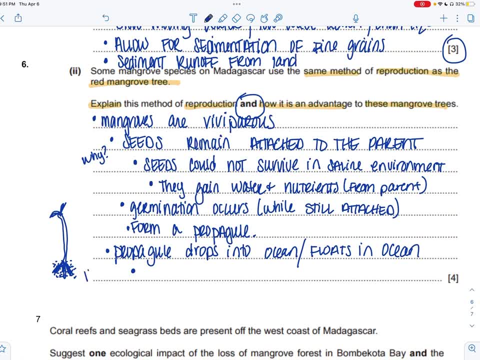 um, i guess, even with just some more detail, like oh how, um, by ocean currents, and not even just the ocean but water currents in general, because you can also have currents from wind and from tidal influence and like the lagoon we live by the indian river lagoon, almost done. 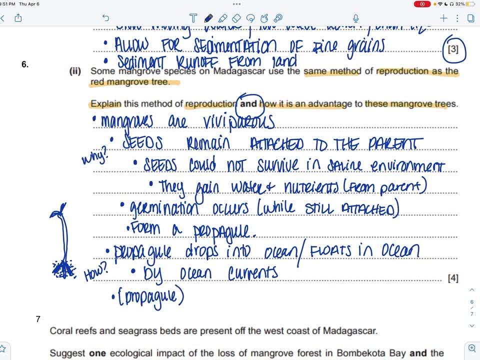 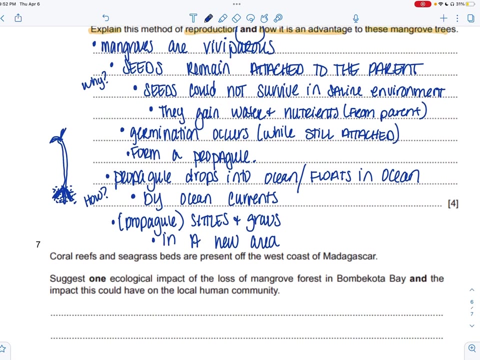 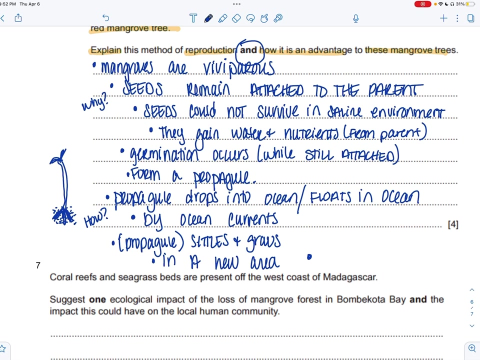 propagule settles and grows in a new area because it's away from the parent plant, and that's the last thing that we can mention. um last mark, the seeds or the propagules move away, or that kind of statement to not, and by the move you can all say float. 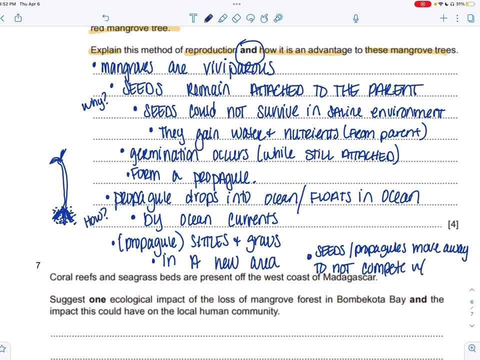 compete with the parent plant, and so that's the last thing that we can mention about the parent plant, and so that's the last thing that we can mention about the parent plant, and so that's the last thing that we can mention about the parent plant. and so it's effective that they move so far away and they can. 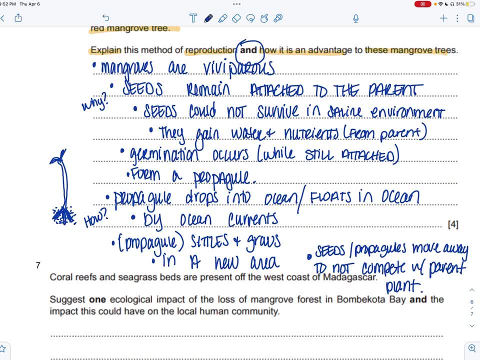 you know, float on average for 40 days, but they can float all the way up to a whole year. and then, finally, when they find some soft sediment, like a soft sandy substrate or muddy substrate, they will embed themselves in it. they'll just land in it, they'll settle in it and start to grow. 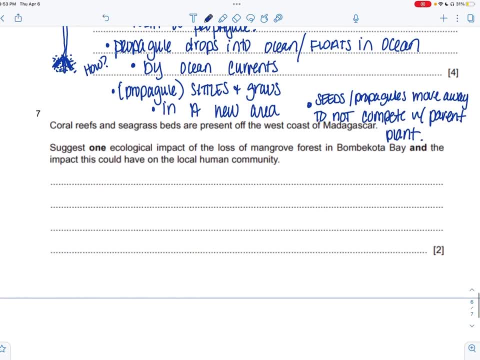 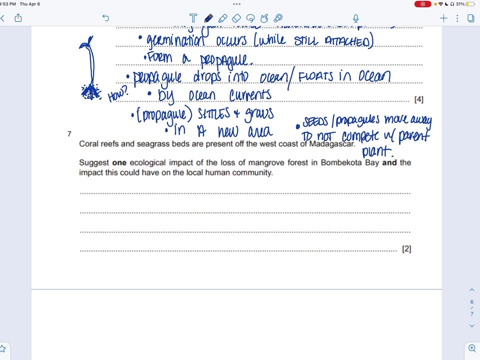 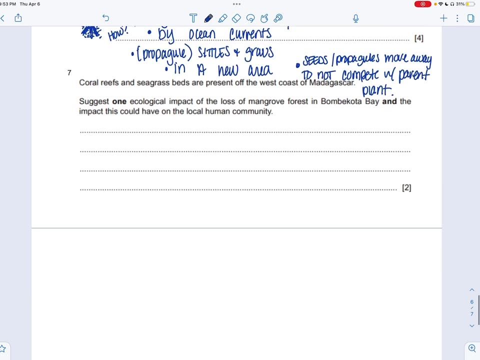 the roots. last one: this one is. this one is interesting. i had to look at it a handful of times just to make sure that i could answer it correctly and just make sense of it. okay, one of the other things mentioned in the notes is that coral reefs and mangroves go really well together. 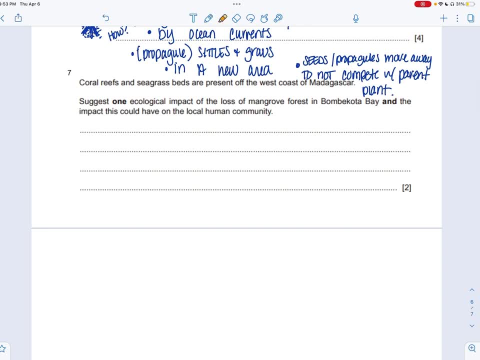 not just that, but mangroves will also assist in stopping the deposition or the sedimentation of fine sediments on coral reefs by slowing down the water first and trapping sediments. you don't want it to land in a coral polyp and then have it block the coral polyp from being able to feed. 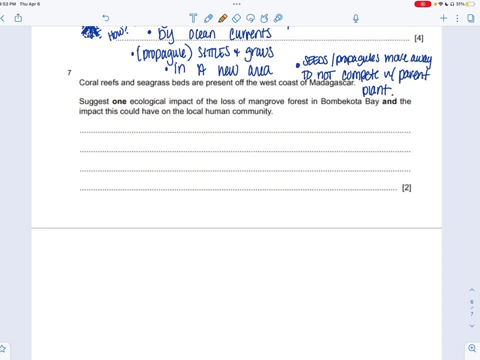 also from blocking sunlight penetration to the zozan valley, then for other species that would be able to spawn some of those tãoih while they're still growing, also from blocking sunlight penetration to the zozan valley, then for other species that would be able to spawn some of those tanih while they're still growing. 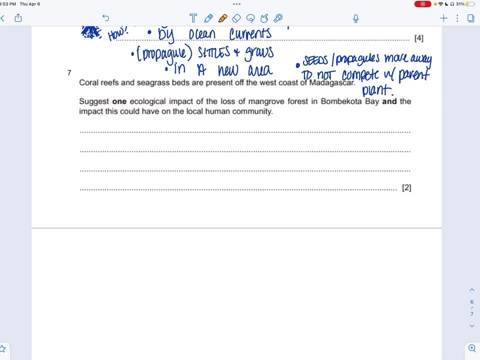 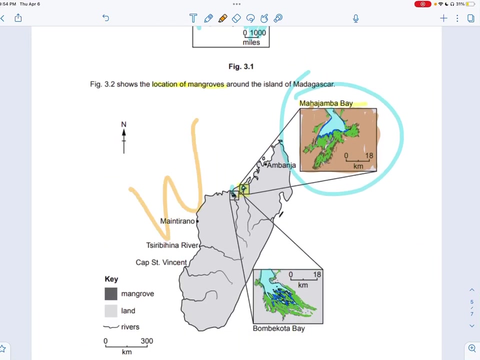 lives in the coral tissues. likewise, sediment can land on the seagrass beds and kind of start to bury the seagrasses. coral reefs and seagrasses are seagrass beds, are both present off the west coast of madagascar and that was on the map here. this is the west coast. 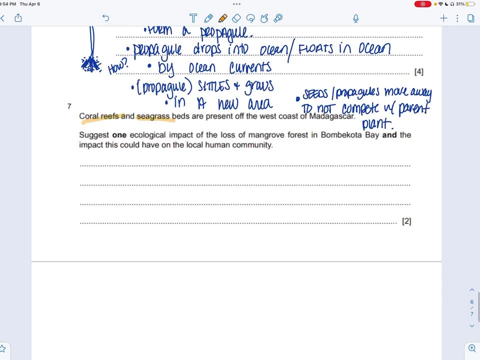 suggest one ecological impact of the loss of a mangrove forest in the bombicota bay, one ecological impact, so something that's happening to the ecosystem and so that will give you the one mark, the impact this would have on the local human community. so it can't be separate, they need to be linked together. so the 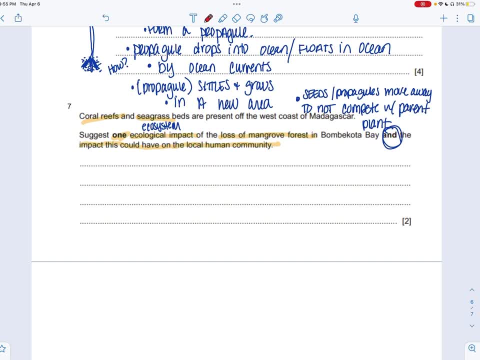 ecological impact caused because of the mangrove loss and the impact that, whatever you just stated, the ecological one. this this meaning the ecological impact, how that would affect a human community. it's our last question. all right, we can start with the the obvious, because they did mention. 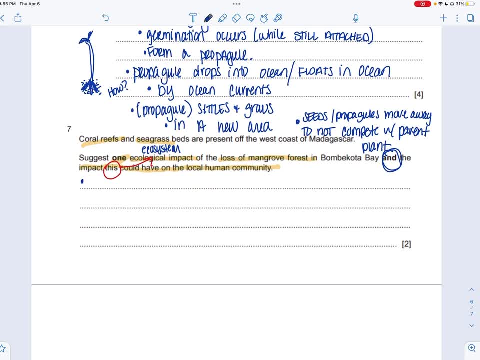 coral reefs and seagrass beds. so this is going to be referencing these marks i'm going to give. here is loss, mangrove, impact on ecosystem, and there will be a few of them. build up sediments on a coral reef or the seagrass bed itself. 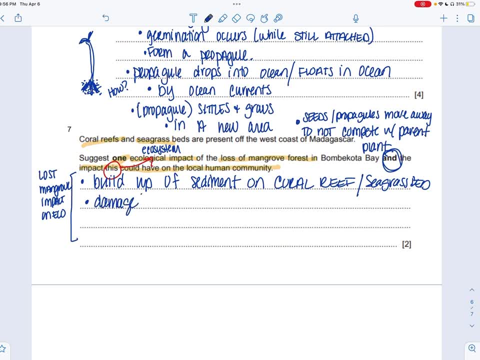 referencing damage or loss to the nursery area from mangroves or nursery area areas for fish for marine species. this is where juveniles hang out until they're adults, and then they can go to the ocean within this same mark. this is where a whale might be somewhere else if they're in the same species of a marine species or any facility. but don't look at them ourselves. 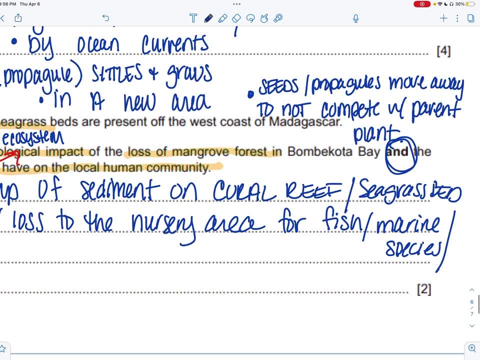 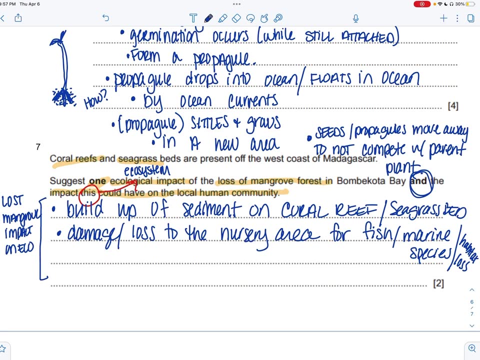 Within this same mark- I'm going to squeeze it in- We're talking about nursery area loss or damage. This can also talk about habitat loss for marine species or fish, Because then that's going to be an easy link to humans, because that's a food source for us. 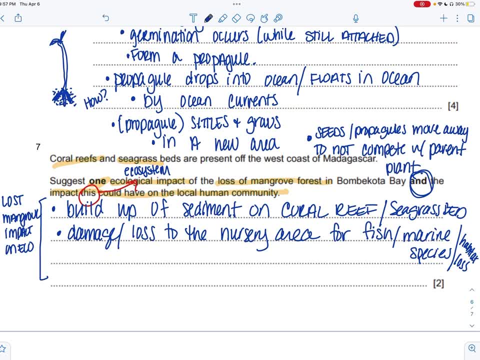 And it's also something that we can make money off of. Okay, you can also talk about biodiversity loss, And so biodiversity- remember it- has three different components to it: The genetic diversity, the species diversity and the ecosystem diversity. So you're going to lose the different ecosystems. 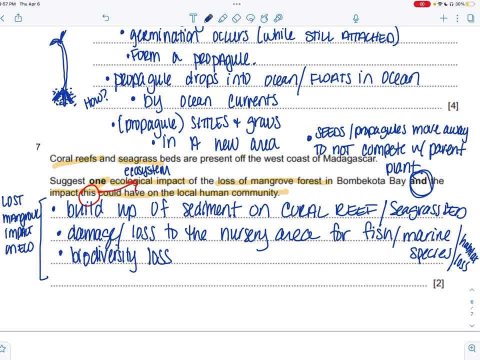 You're going to lose the different species there, And, because different species aren't going to be living there and you're not going to have so many niches for them to be able to accommodate and take advantage of, you're going to then lose the overall variations in your gene pool. 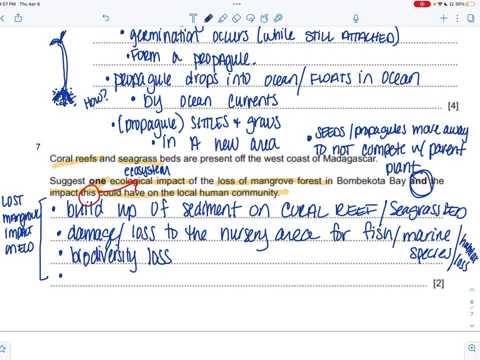 And the last one: water quality loss. Remember, mangroves filter out like impurities in the water, So this would be the impact on ecosystems if you had loss of a mangrove forest, And so you would just need one of these. 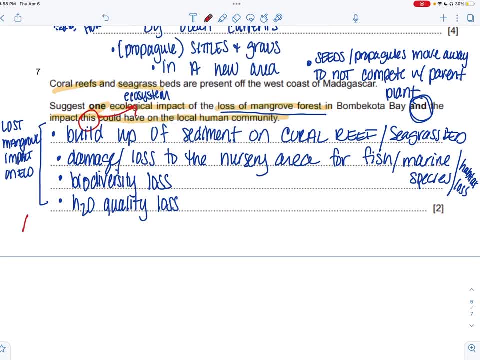 And How one of these things will affect the human. I'll do the human one in purple. So this is going to be the human impact. I don't like the way that sounds. Impact on human community is better. Human impact makes it seem like humans did this. 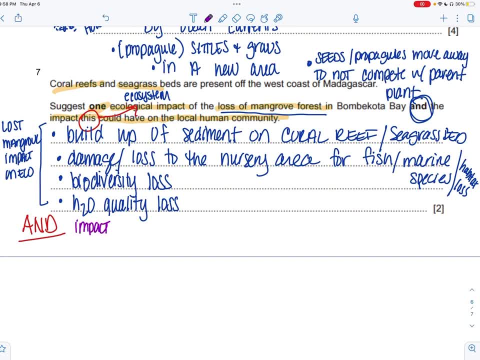 Although humans probably did, They're probably the cause of the loss of the mangrove forest Impact on human community. Okay, So you could say this could cause a decrease in fish population. That one would be pretty direct with the damage loss to nursing homes. 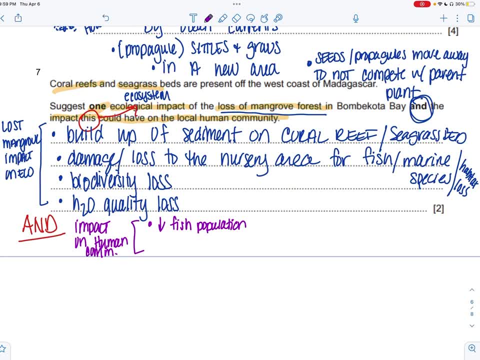 Can you tell the resource that this is going to affect the ecosystem? This is probably the most important thing that you can think about And making sure that you're okay with just giving and then if it's a generic resource, and then maybe there's other sources you can use. 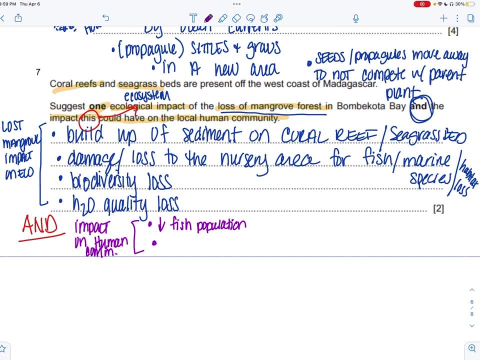 Just look at it. If it's a terrestrial resource you're going to think about, hey, maybe that could play a role in reducing biodiversity loss, but you're in a very diverse area for fish or marine species or habitat loss. Additionally, 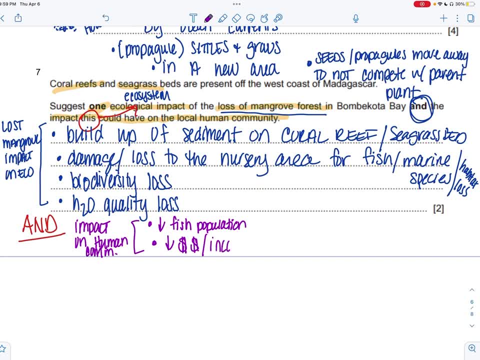 that goes with biodiversity loss but also go with water quality loss, And you only need one. You actually can only put one: One of the ecosystem impact and then one of how that's going to affect human communities. Decrease Money or income from fishing. 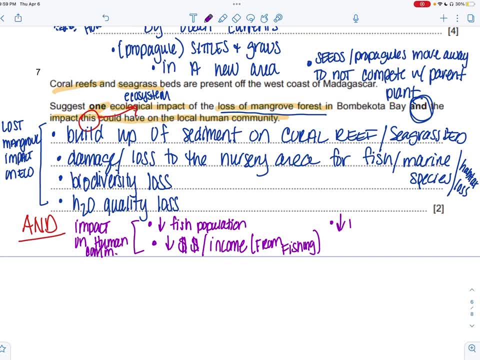 And that's kind of the bowl with the quiver or whatever else. decrease fish catches or fish harvests because there's not as much there. Again, that's a food source for us, So it's impact on humans. I think if you were going to say decrease in a food source, 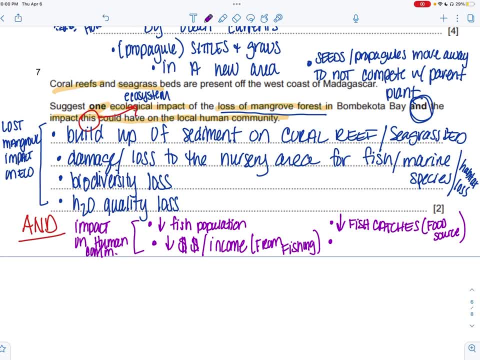 I would just maybe reference to like decrease on fish as a food source or lack of that, And decrease in tourism, because nobody wants to go to a place that's not going to be as biodiverse and doesn't have the same amount and variety of organisms. 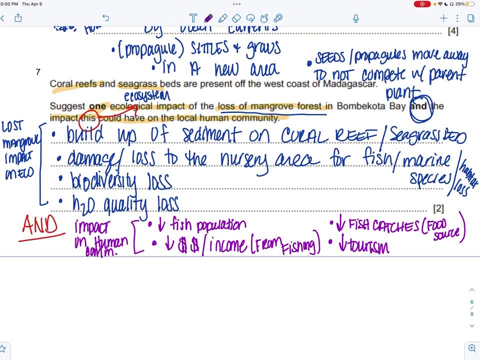 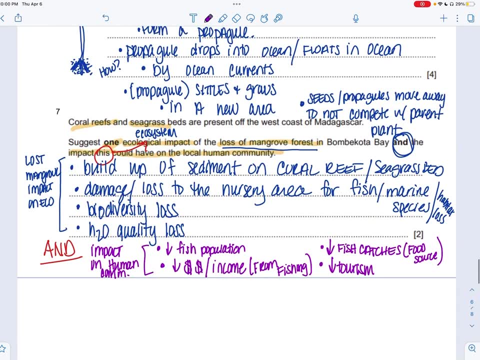 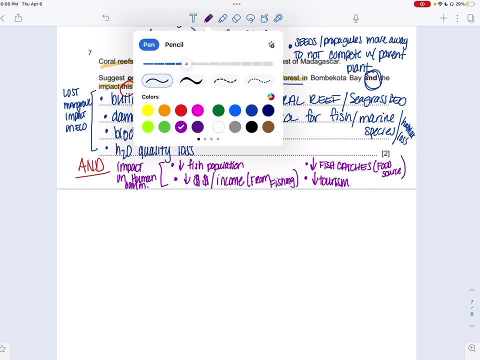 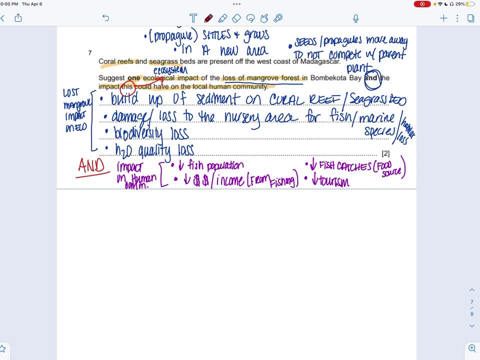 It could be that on the ecosystem, you're going to have a decreased protection of the shoreline. The shoreline isn't just necessarily for humans, right? We have sand dunes there, We have nesting turtles, sea turtles. We have marine birds. 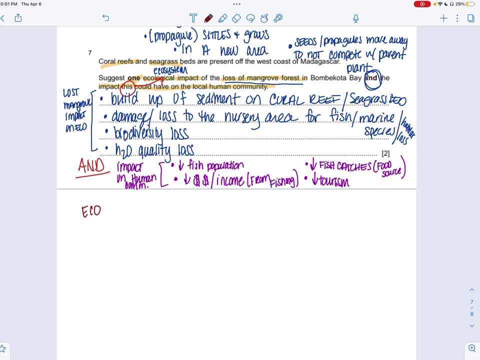 So this is another option If you're going this route. the one I just put like what we wrote in purple is very specific to everything that was in blue. For this one, the ecosystem or ecological impact impact on that ecosystem could be decreased. protection off shorelineses and for the human. 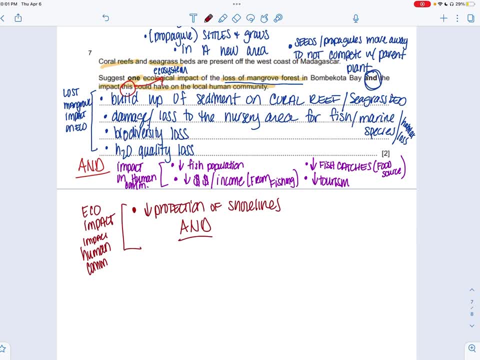 community. impact on human community. this is going to be terrible for us. um, this is going to increase coastal erosions, could increase flooding. all right, so there you go. those are the mangrove questions, and you're so close to your exam, good job for going this whole way. uh, despite me chatting it up and all that, it's really really. 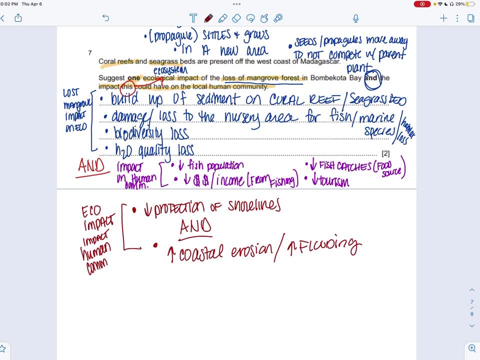 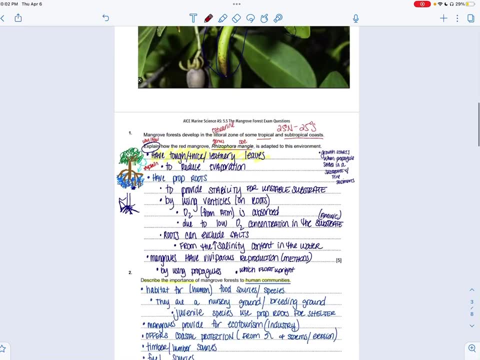 really great review for you guys to see and talk out and make, try and make sense of the mark scheme, and you also got to add a couple extra details that you could put on your note sheet, mainly that mangroves have very tough, thick and leathery leaves. enjoy your long weekend and thanks. 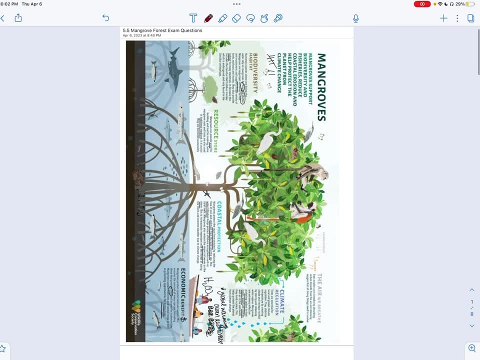 for doing this and you're gonna do great. in what 17 days? if you're watching this, tomorrow, saturday, it's tomorrow friday, 16 days, yikes. okay, guys, have a good night. 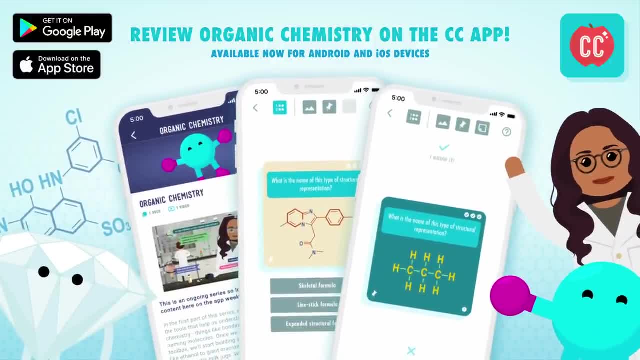 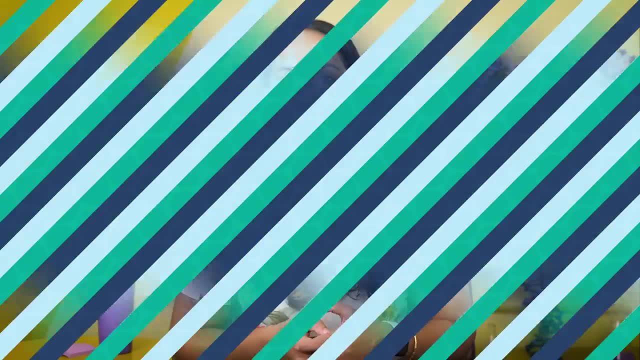 You can review content from Crash Course Organic Chemistry with the Crash Course app, available now for Android and iOS devices. Hi, I'm Deboki Chakravarty and welcome to Crash Course Organic Chemistry. When you buy a new TV or some bulky kitchen gadget, 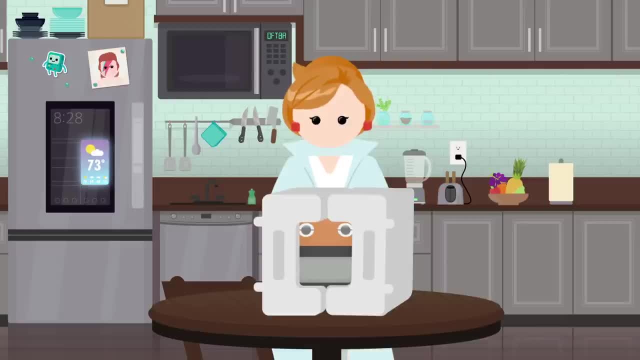 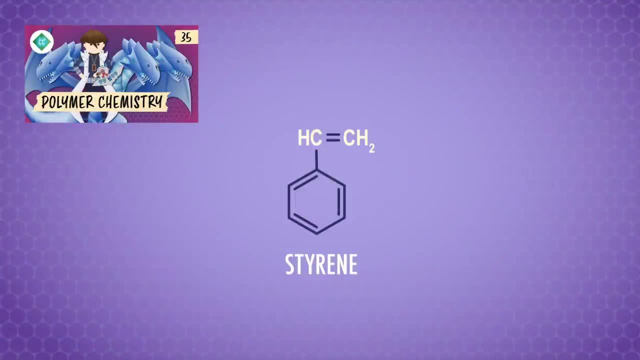 it often comes packed in that white solid foam stuff that can make a horrible squeaky noise. That's polystyrene, which we met in episode 35 on polymers. There we saw that polystyrene is made by joining together lots of styrene monomers. 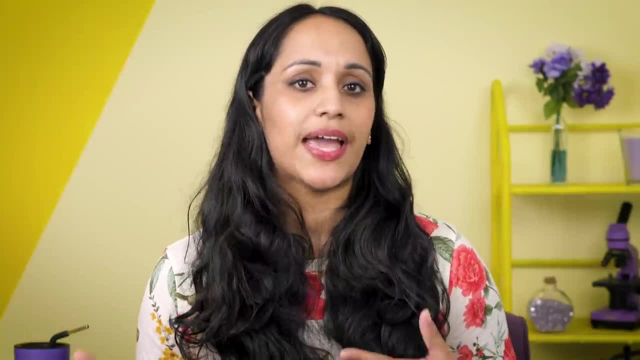 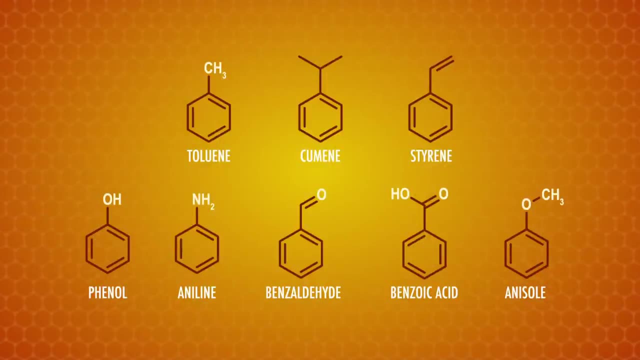 By the way, you can name these substituted benzenes with the IUPAC rules. we learned before, but many of them have been known for a long time. So styrene isn't just the historical common name, it's also IUPAC official.